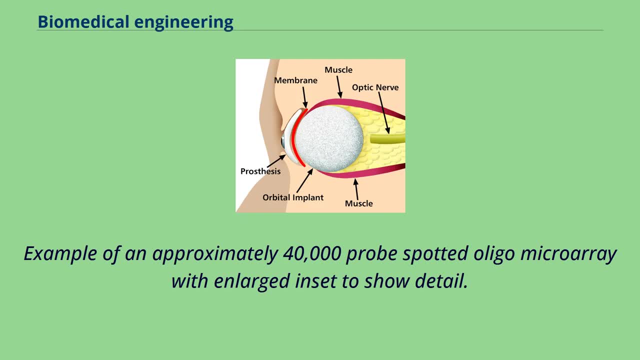 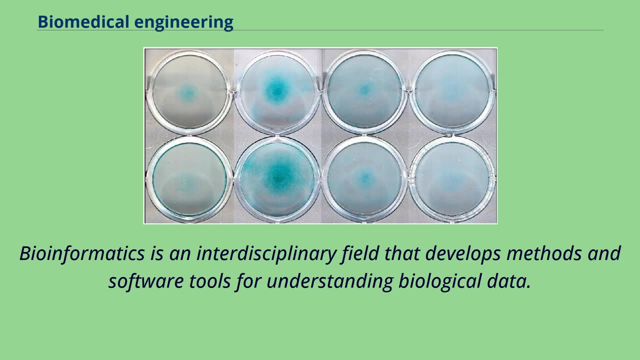 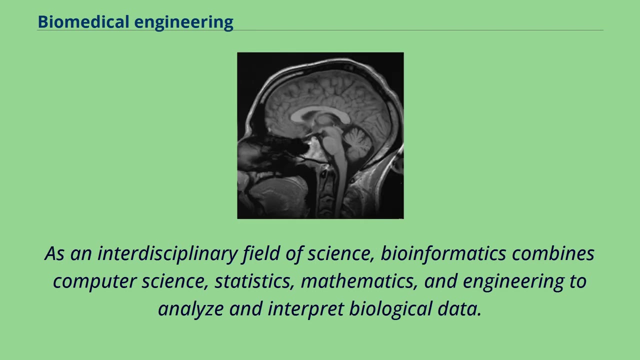 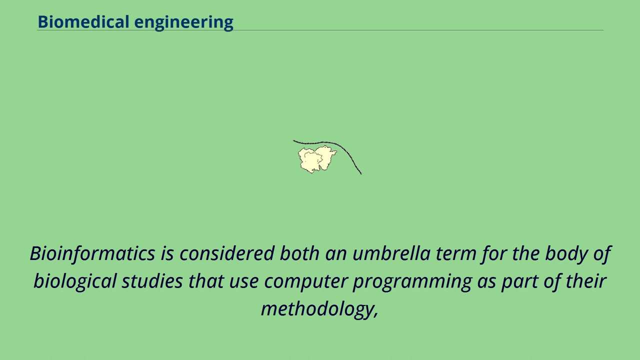 pharmaceutical drugs and therapeutic biologicals. Example of an approximately 40,000 probes spotted oligo-microarray with enlarged inset to show detail. Bioinformatics is an interdisciplinary field that develops methods and studies to improve the quality of medical equipment. Bioinformatics is considered both an umbrella term for the body of biological studies that use 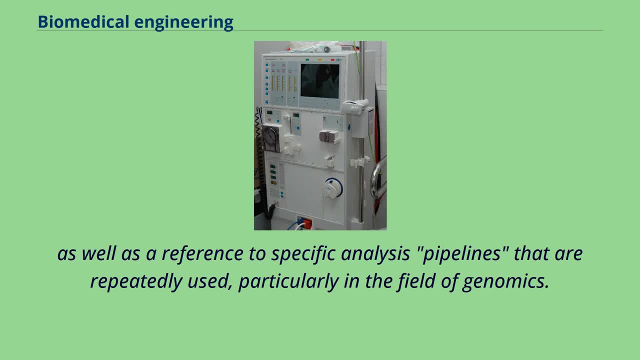 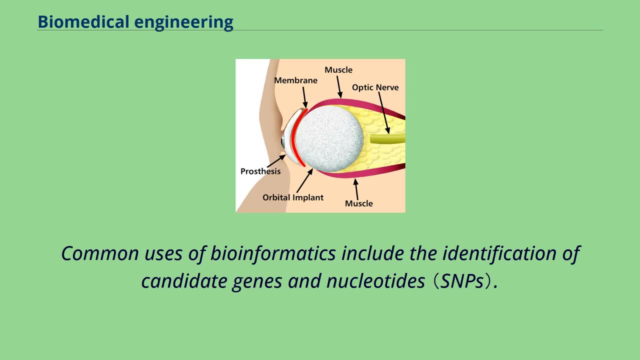 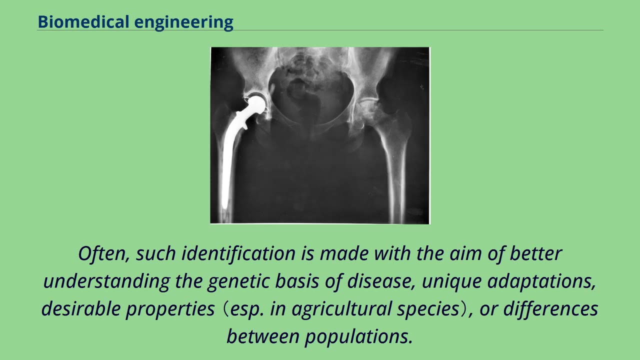 computer programming as part of their methodology, as well as a reference to specific analysis pipelines that are repeatedly used, particularly in the field of genomics. Common uses of bioinformatics include the identification of candidate genes and nucleotides. Often, such identification is made with 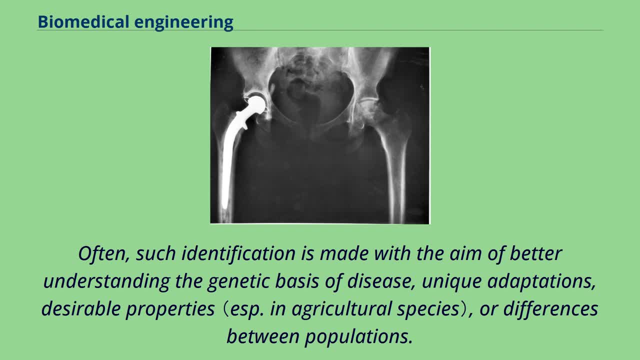 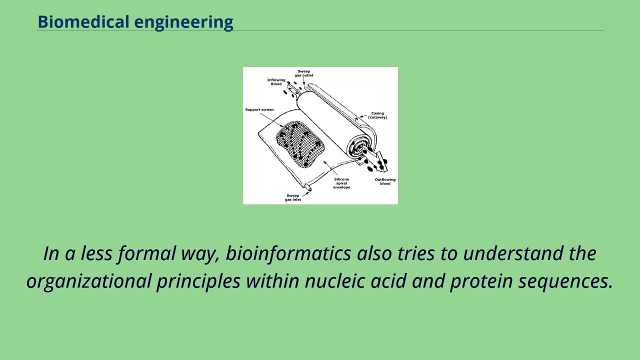 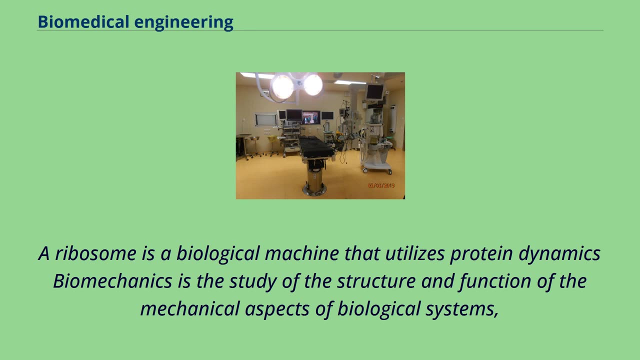 the aim of better understanding the genetic basis of disease, unique adaptations, desirable properties or differences between populations. In a less formal way, bioinformatics also tries to understand the organizational principles within nucleic acid and protein sequences. A ribosome is a biological 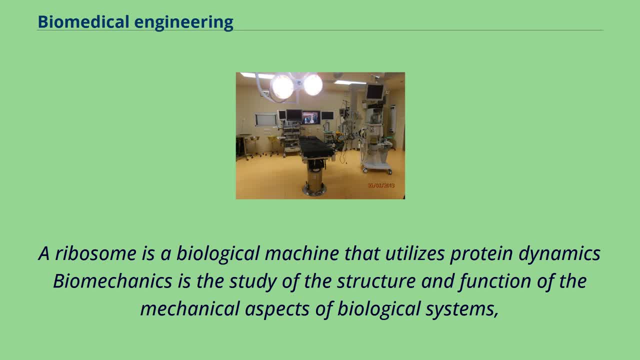 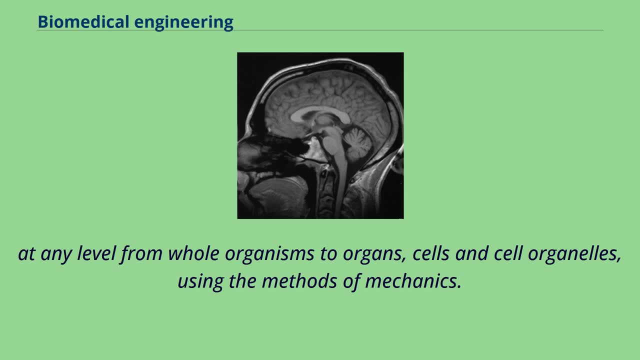 machine that utilizes protein dynamics. biomechanics as the study of the structure and function of the mechanical aspects of biological systems At any level, from whole organisms to organs, cells and cell organelles, using the methods of mechanics. A biomaterial is any matter. 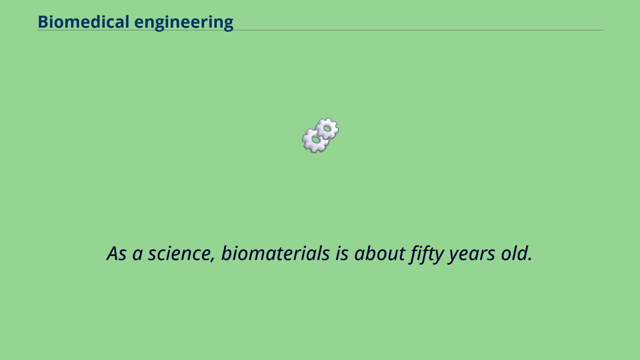 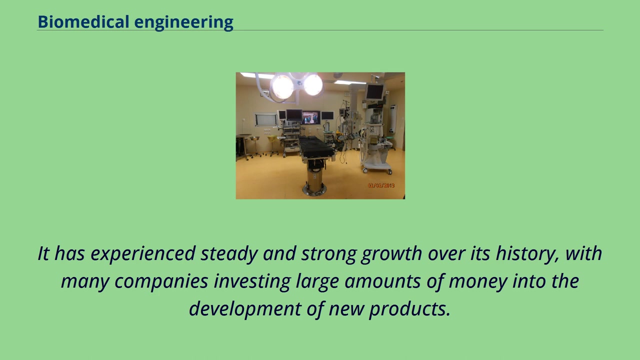 surface or construct that interacts with living systems. As a science, biomaterials is about 50 years old. The study of biomaterials is called biomaterials science or biomaterials engineering. It has experienced steady and strong growth over its history, with many companies investing large. 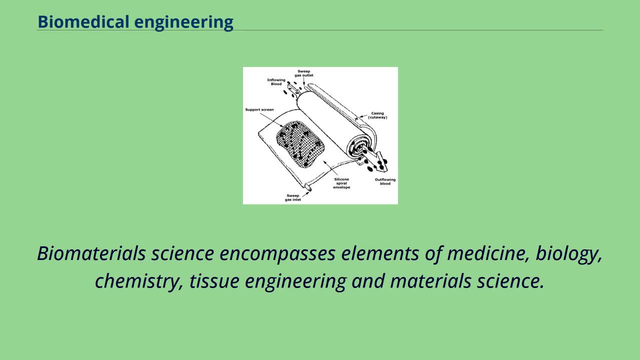 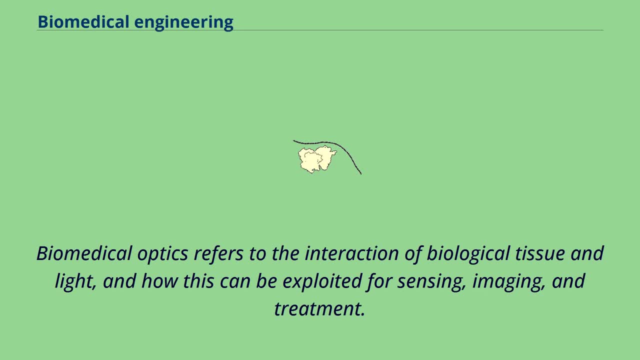 amounts of money into the development of biomaterials. The study of biomaterials is of new products. Biomaterials science encompasses elements of medicine, biology, chemistry, tissue engineering and materials science. Biomedical optics refers to the interaction of biological tissue and light and how this can be exploited for sensing, imaging and treatment Tissue. 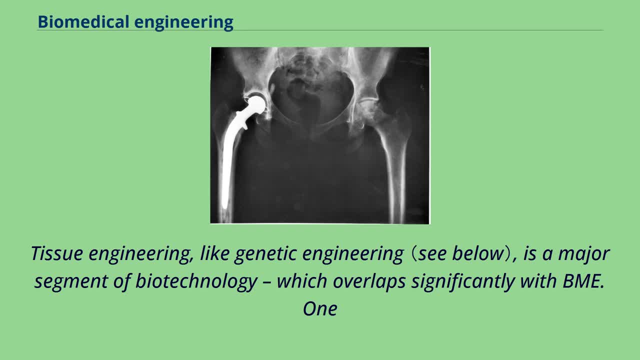 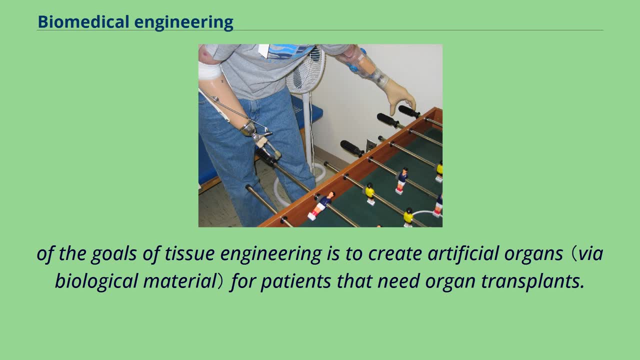 engineering, like genetic engineering, is a major segment of biotechnology which overlaps significantly with BME. 1. Of the goals of tissue engineering is to create artificial organs for patients that need organs. 2. Of the goals of tissue engineering is to create artificial organs for: 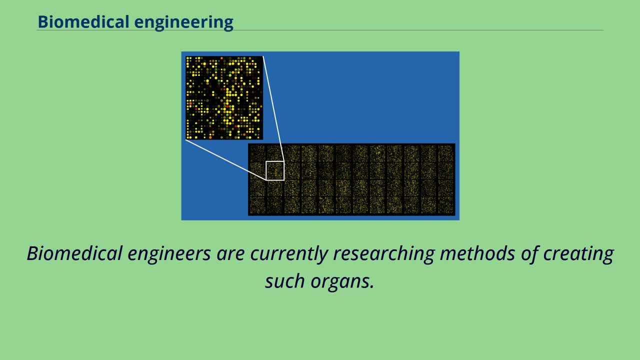 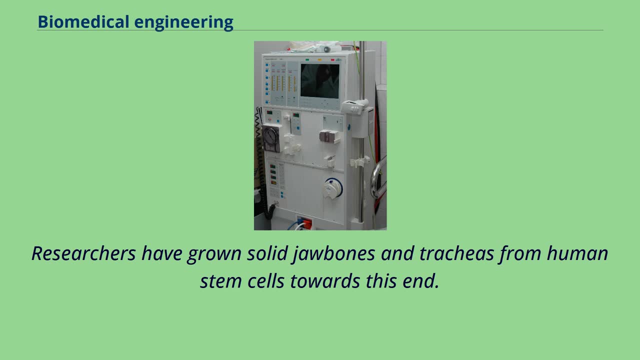 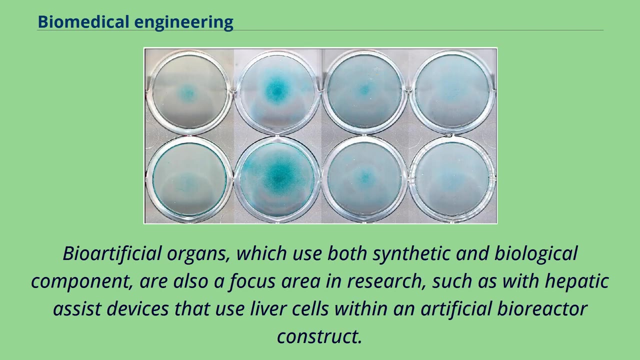 transplants. Biomedical engineers are currently researching methods of creating such organs. Researchers have grown solid jawbones and tracheas from human stem cells towards this end. Several artificial urinary bladders have been grown in laboratories and transplanted successfully into human patients Bioartificial organs which use both. 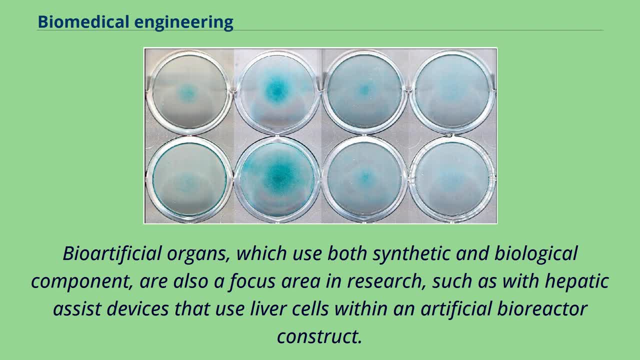 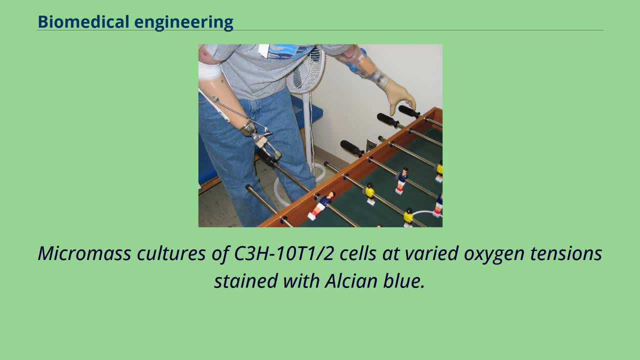 synthetic and biological component are also a focus area in research, such as with hepatic assist devices that use liver cells within an artificial bioreactor, construct Micromask cultures of CHATEN T1-2 cells at varied oxygen tensions stained with alcyon blue. 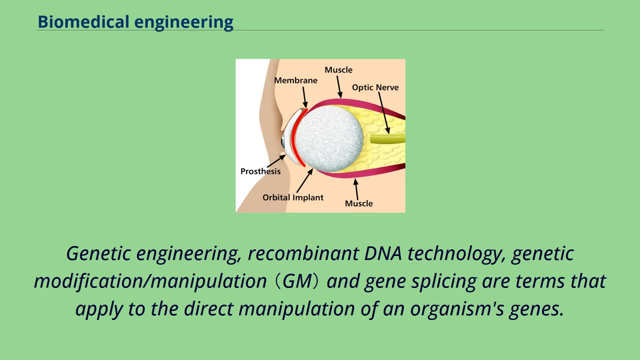 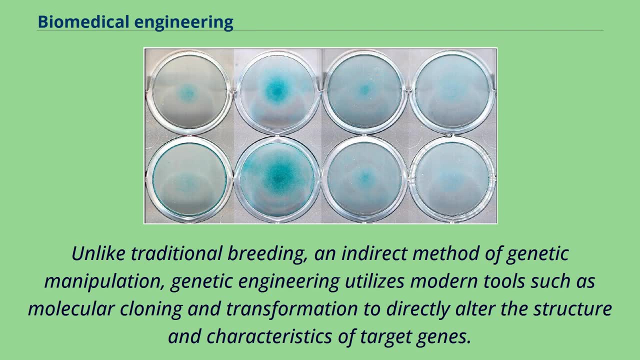 Genetic engineering, recombinant DNA technology, genetic modification-slash-manipulation and gene splicing are terms that apply to the direct manipulation of an organism's genes. Unlike traditional breeding, an indirect method of genetic manipulation, genetic engineering utilizes modern tools such as molecular cloning and transformation. 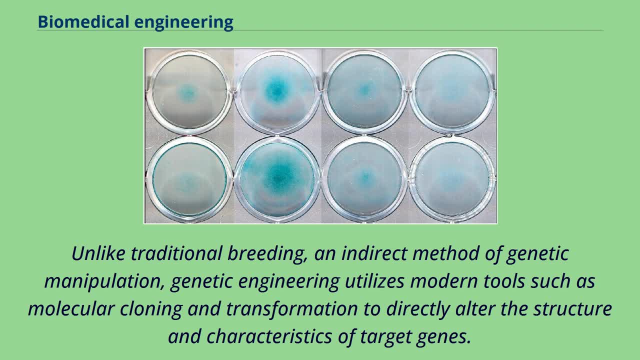 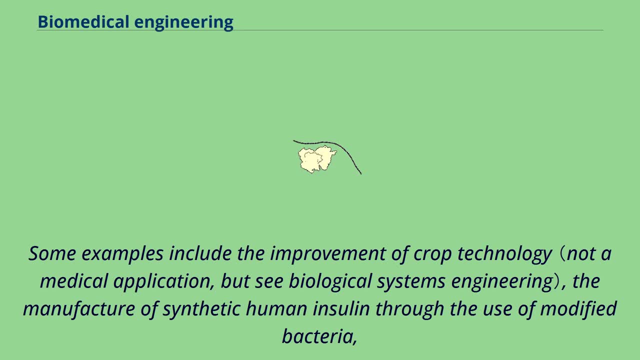 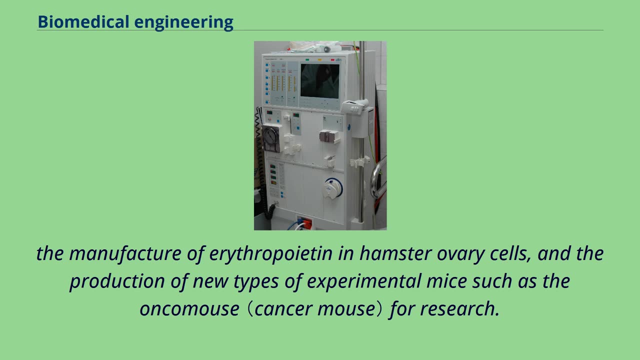 to directly alter the structure and characteristics of target genes. Genetic engineering techniques have found success in numerous applications. Some examples include the improvement of crop technology, the manufacture of synthetic human insulin through the use of modified bacteria, the manufacture of erythropoietin in hamster ovary. 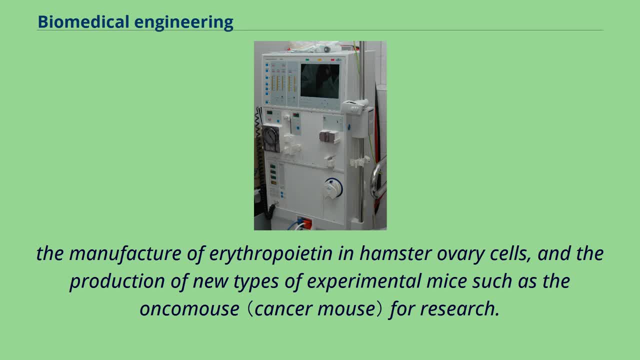 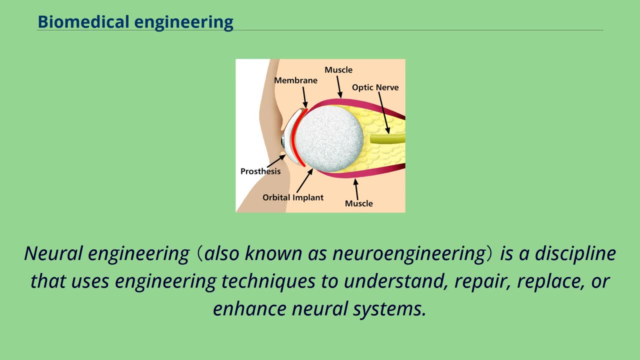 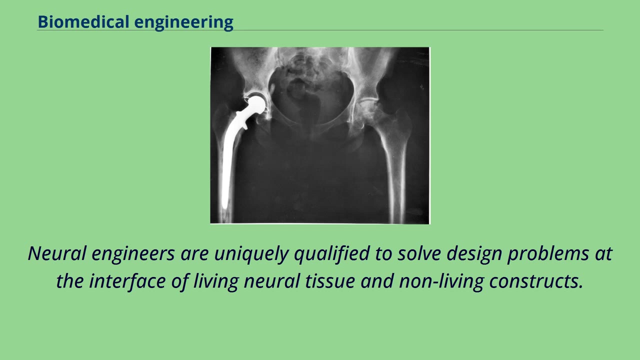 cells and the production of new types of experimental mice, such as the oncomouse for research. Neural engineering is a discipline that uses engineering techniques to understand, repair, replace or enhance neural systems. Neural engineers are uniquely qualified to solve design problems at the interface of living neural tissue and non-living constructs. 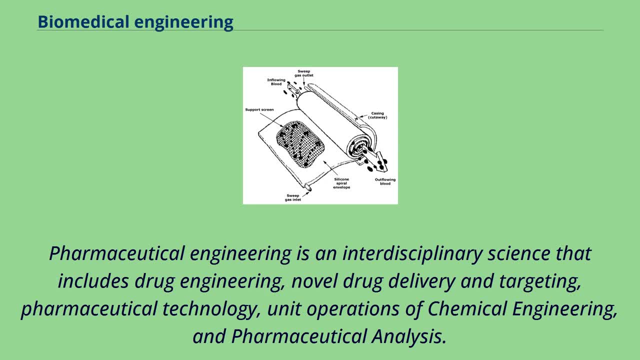 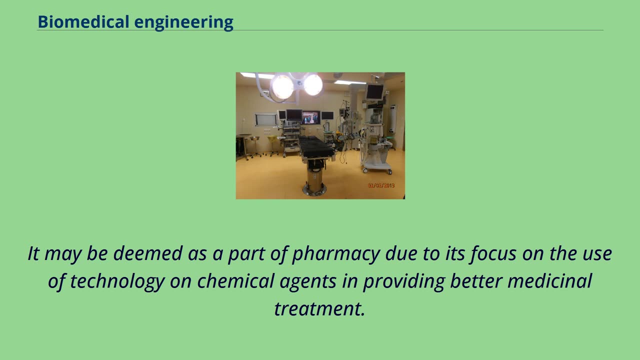 Pharmaceutical engineering is an interdisciplinary science that includes drug engineering, novel drug delivery and targeting pharmaceutical technology unit operations of chemical engineering and pharmaceutical analysis. It may be deemed as a part of pharmacy due to its focus on the use of technology on chemical agents in providing better medicinal treatment. Schematic of silicone membrane. 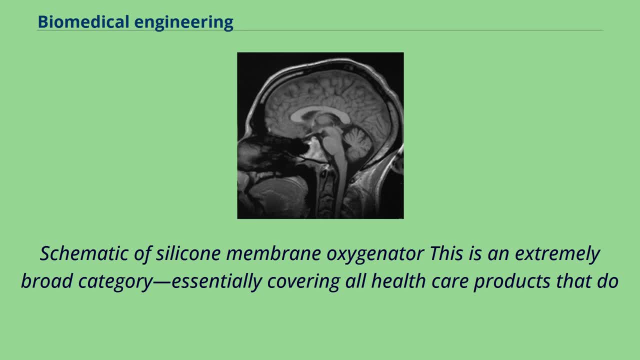 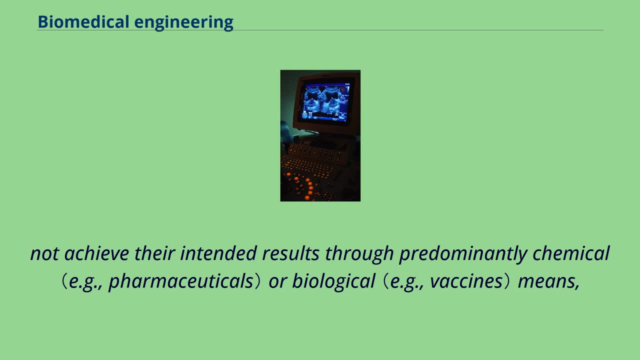 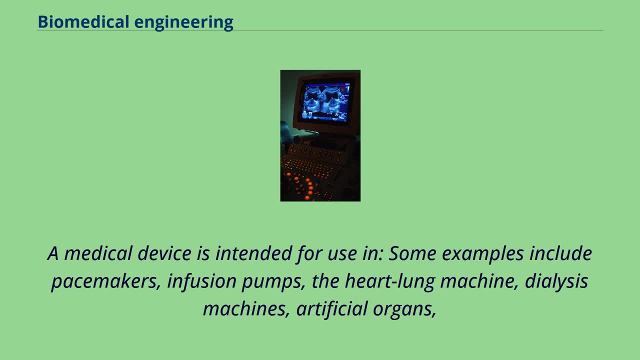 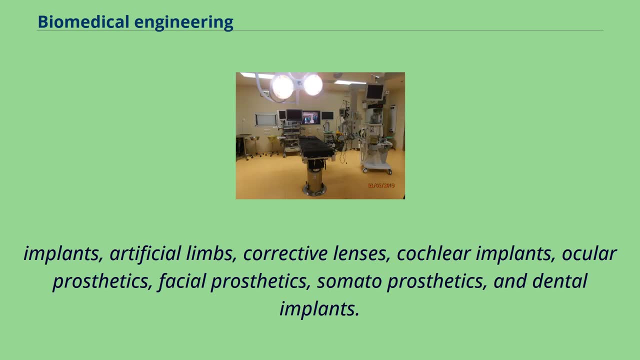 A medical device is intended for use in. some examples include pacemakers, infusion pumps, the heart-long machine, dialysis machines, artificial organs implants, artificial limbs, corrective lenses, cochlear implants, ocular prosthetics, facial prosthetics, somatoprosthetics. 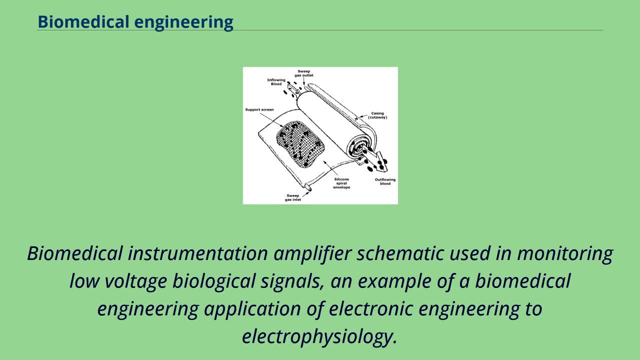 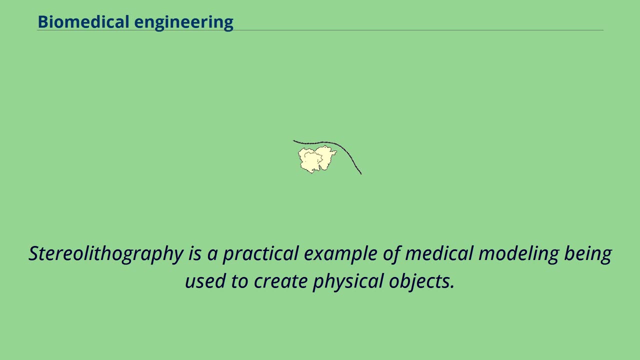 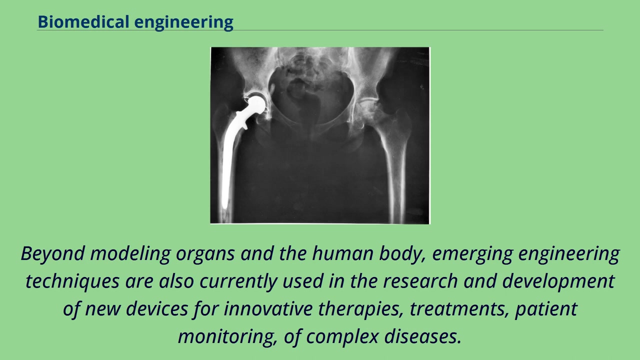 and dental implants. Biomedical instrumentation: amplifier schematic used in monitoring low-voltage biological signals. an example of a biomedical engineering application of electronic engineering to electrophysiology. Stereolithography is a practical example of medical modeling being used to create physical objects. Beyond modeling organs and the human body: emerging engineering. 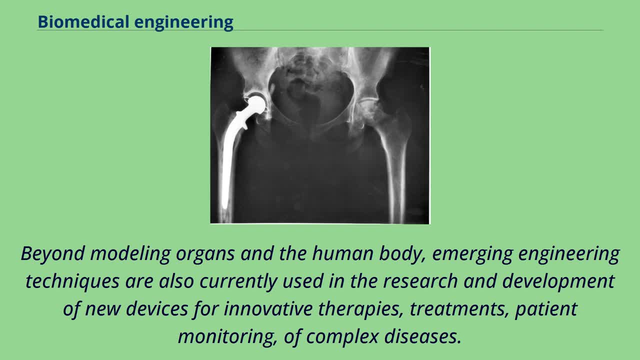 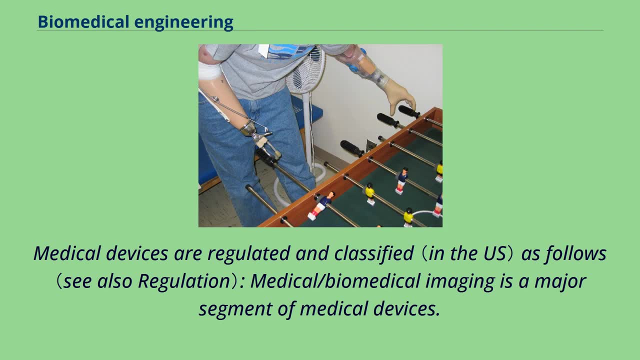 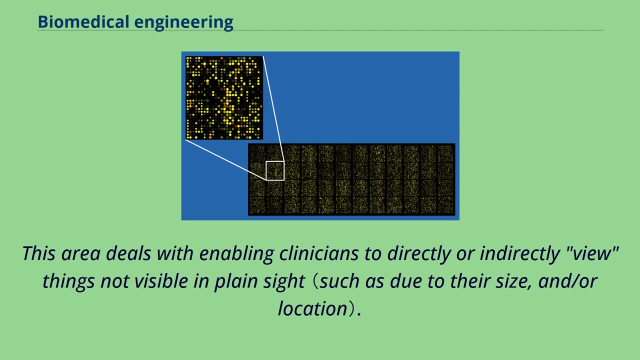 techniques are also currently used in the research and development of new devices for innovative therapies, treatments, Patient Monitoring of Complex Diseases. Medical devices are regulated and classified as follows: Medical-slash-biomedical imaging is a major segment of medical devices. This area deals with enabling clinicians to directly or indirectly 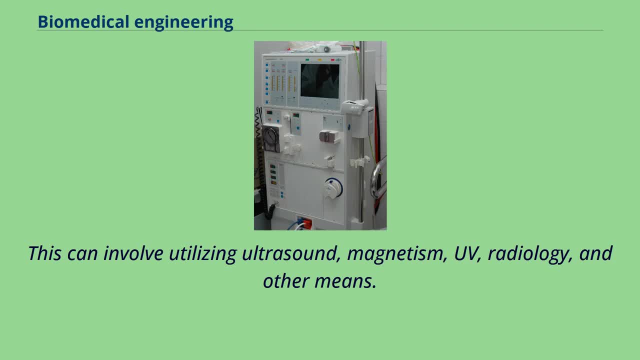 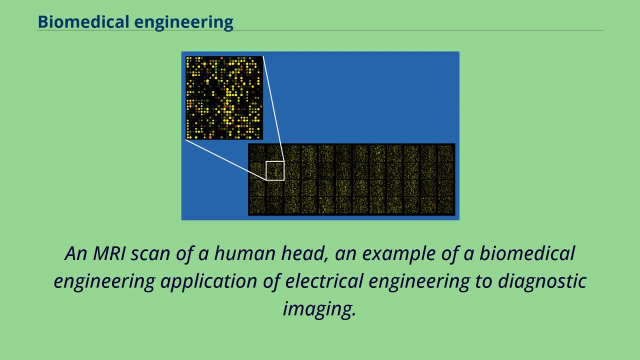 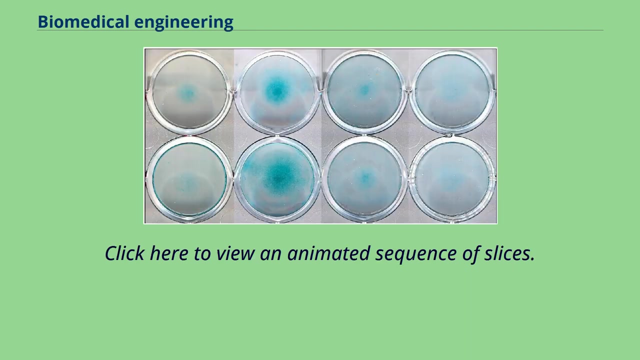 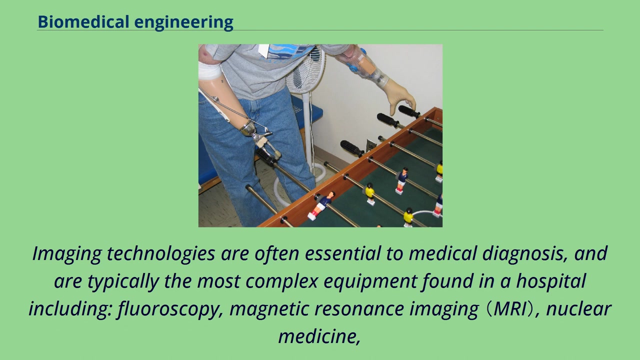 view things not visible in plain sight. This can involve utilizing ultrasound, magnetism, UV radiology and other means. An MRI scan of a human head, an example of a biomedical engineering application of electrical engineering to diagnostic Imaging technologies, are often essential to medical diagnosis and are typically the most 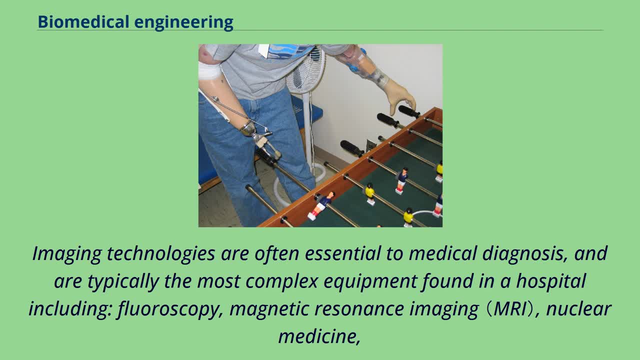 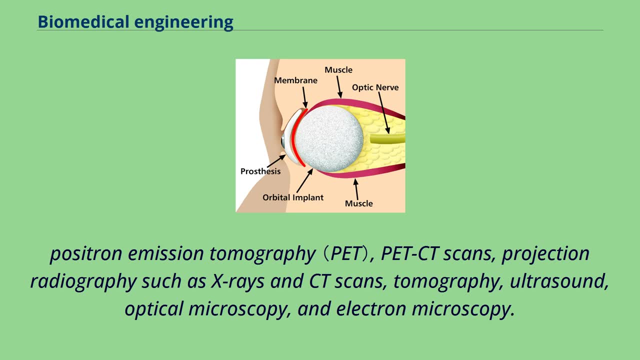 complex equipment found in a hospital, including fluoroscopy, magnetic resonance imaging, nuclear medicine, positron emission tomography, PET-CT scans, projection radiography such as x-rays and CT scans, tomography, ultrasound, optical microscopy and electron microscopy. An implant is a kind of 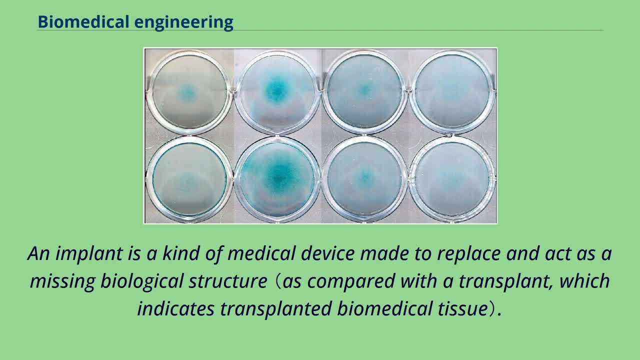 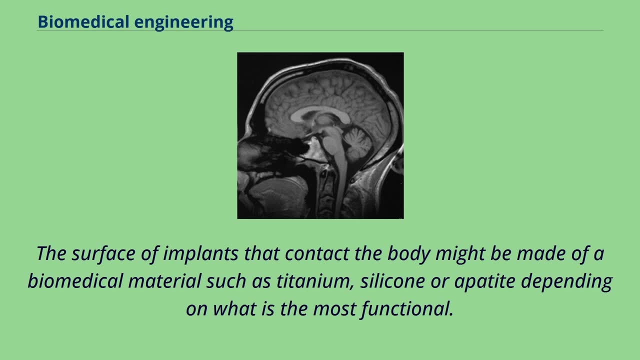 medical device made to replace an implant. An implant is a kind of medical device made to replace and act as a missing biological structure. The surface of implants that contact the body might be made of a biomedical material such as titanium, silicone or apatite, depending on what is the most. 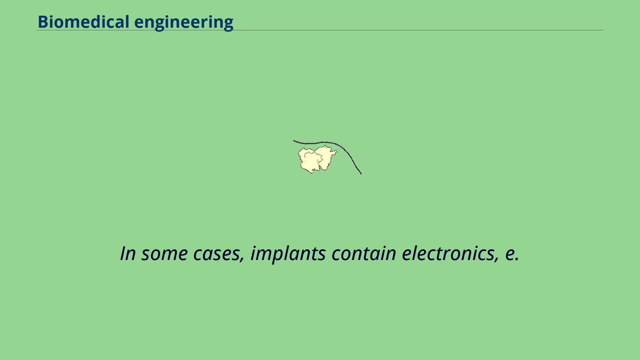 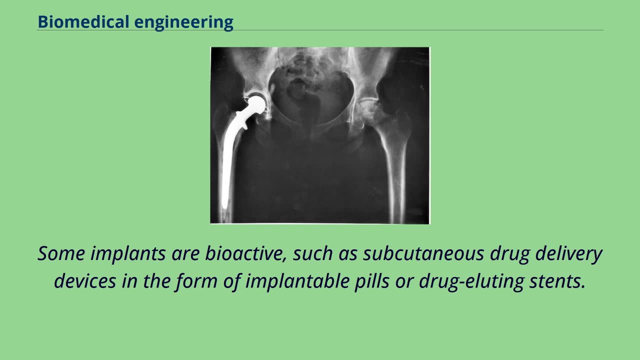 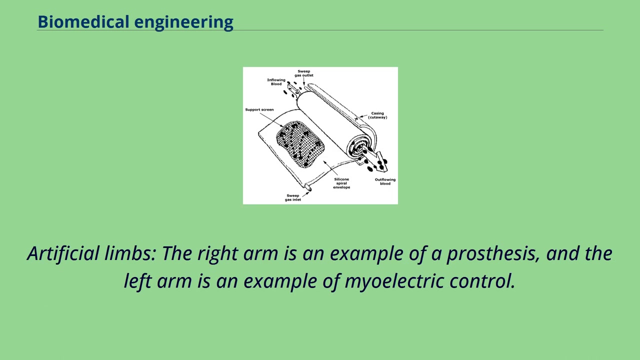 functional. In some cases, implants contain electronics, eg artificial pacemakers and cochlear implants. Some implants are bioactive, such as subcutaneous drug delivery devices in the form of implantable pills or drug-eluting stents. Artificial limbs- the right arm is an. 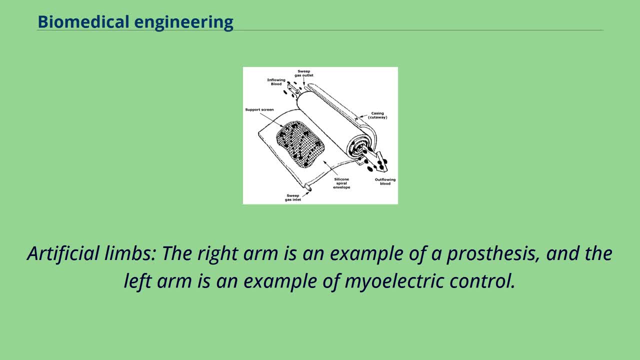 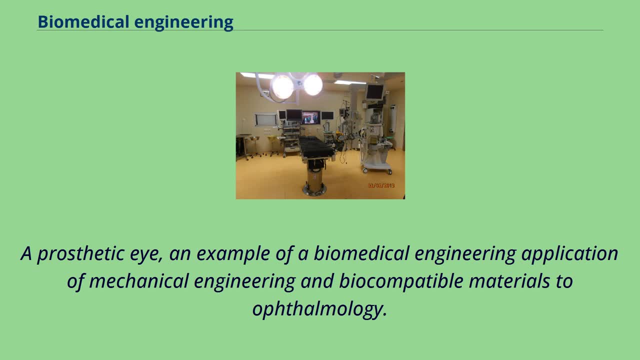 example of a product that can be used to treat an implant. An implant is a kind of medical device, and the left arm is an example of myoelectric control, A prosthetic eye an example of a biomedical engineering application of mechanical engineering and biocompatible materials to 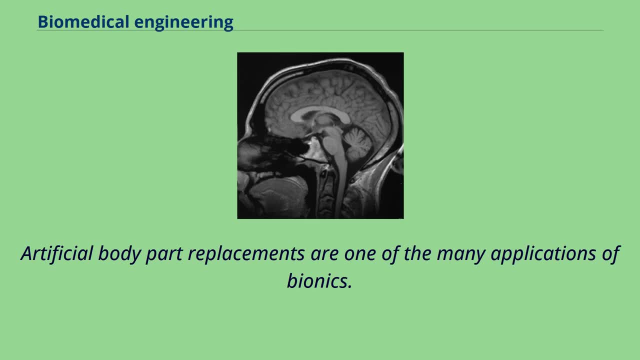 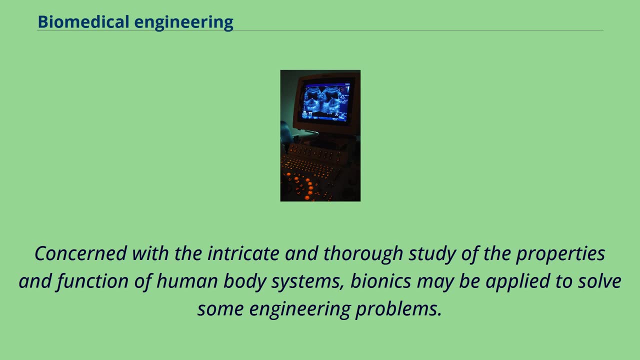 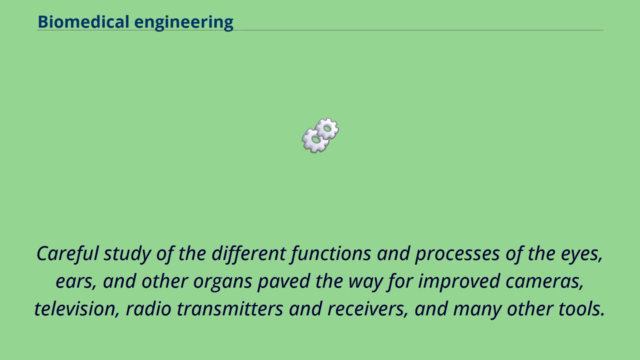 ophthalmology. Artificial body part replacements are one of the many applications of bionics Concerned with the intricate and thorough study of the properties and function of human body systems. bionics may be applied to solve some engineering problems: Careful study of the different functions and processes of the eyes, ears and other. 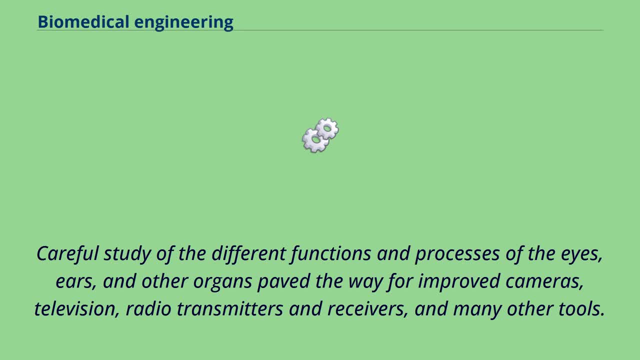 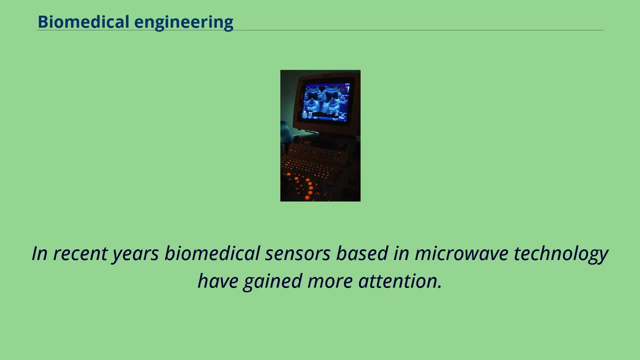 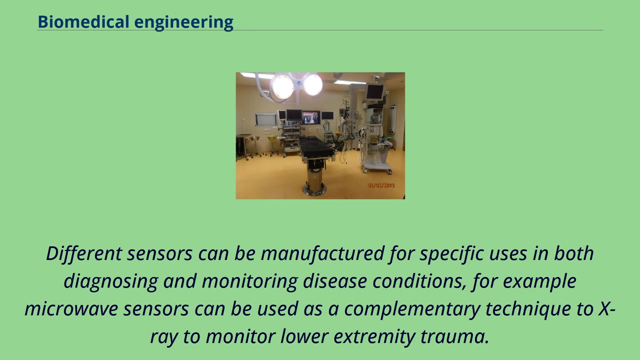 organs pave the way for improved cameras, television radio transmitters and receivers and many other tools. In recent years, biomedical sensors based in microwave technology have gained more attention. Different sensors can be manufactured for specific uses in both diagnosing and monitoring disease conditions. for example, microwave sensors can be used as: 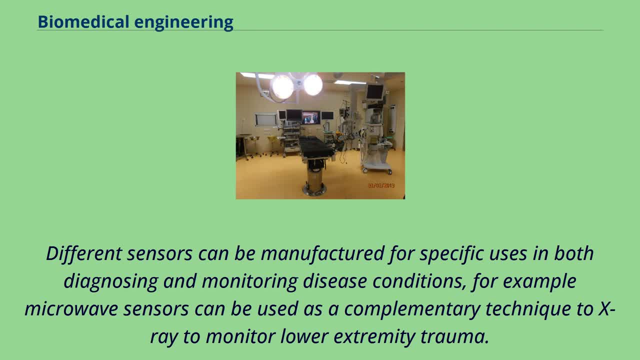 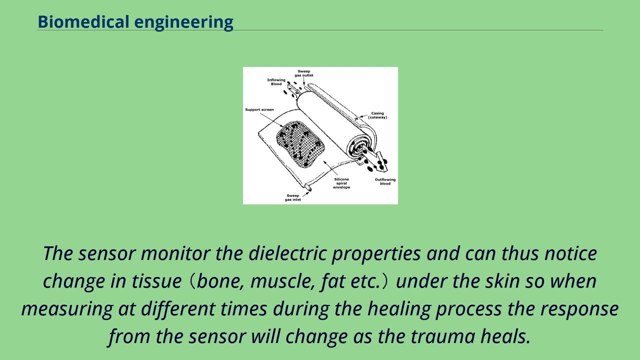 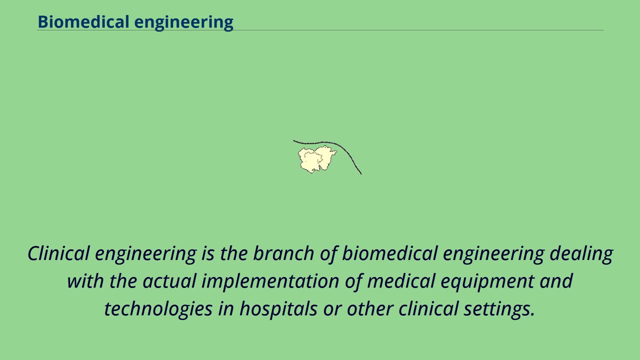 a complementary technique to x-ray to monitor lower extremity trauma. The sensor monitor the dielectric properties and can thus notice change in tissue under the skin. so when the skin is measuring at different times during the healing process, the response from the sensor will change as the trauma heals. Clinical engineering is the branch of biomedical engineering dealing with the 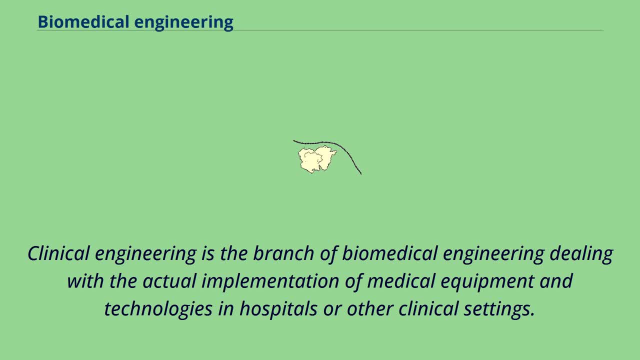 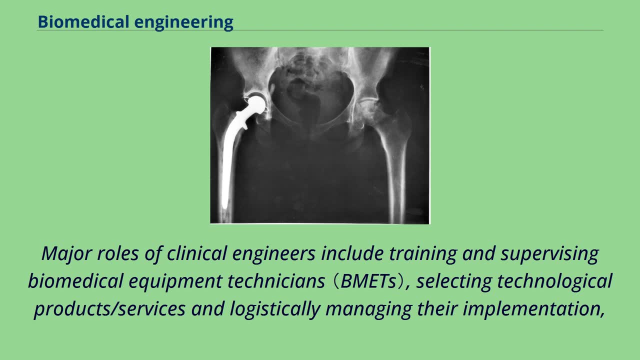 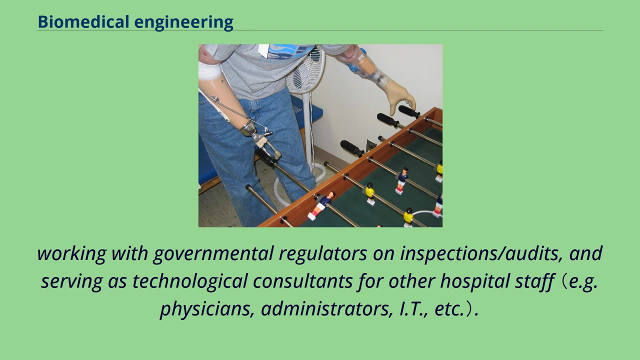 actual implementation of medical equipment and technologies in hospitals or other clinical settings. Major roles of clinical engineers include training and supervising biomedical equipment technicians, selecting technological products, slash services and logistically managing their implementation. Working with governmental regulators on inspections, slash audits and servicing medical equipment is a key part of biomedical engineering. 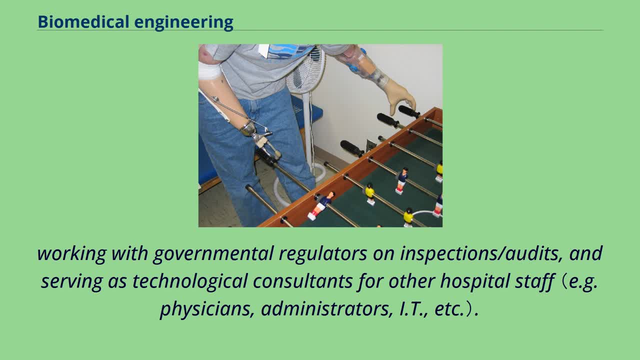 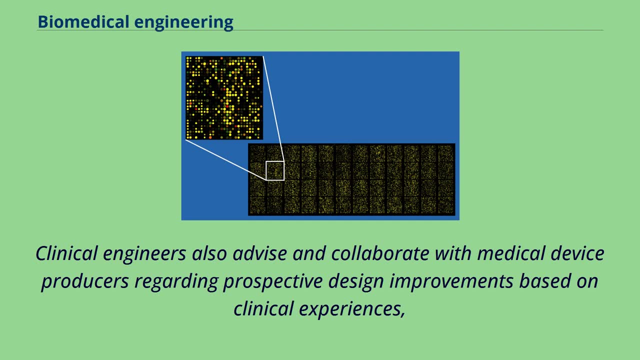 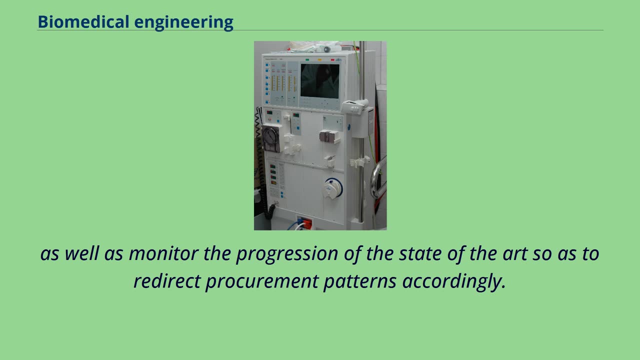 Technical engineers also advise and collaborate with medical device producers regarding prospective design improvements based on clinical experiences, as well as monitor the progression of the state of the art so as to redirect procurement patterns accordingly. Their inherent focus on practical implementation of technology has tended to keep them oriented more towards incremental. 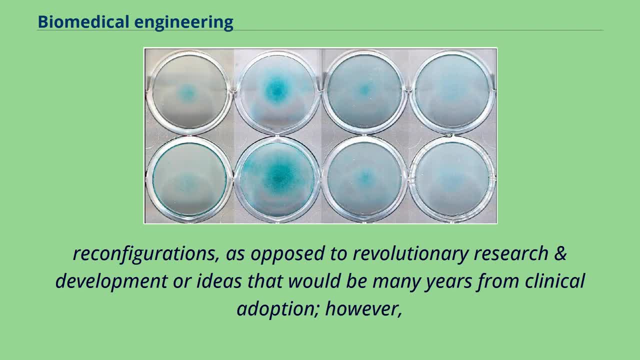 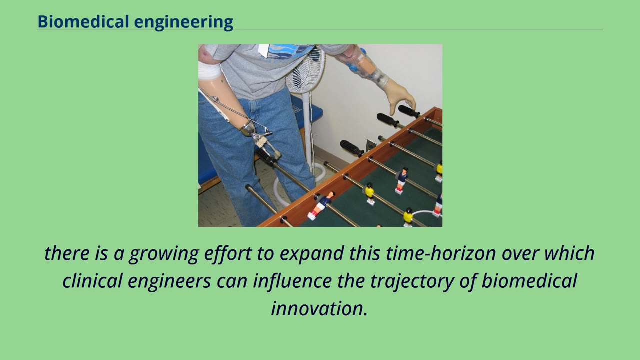 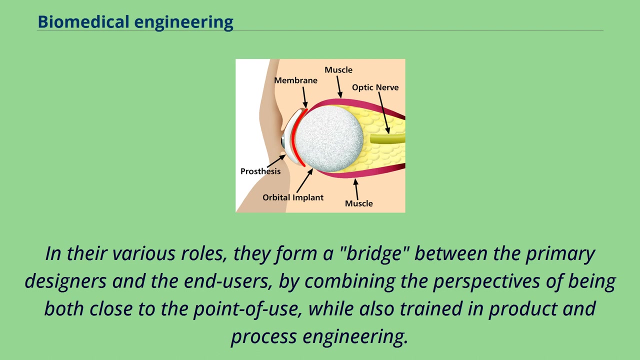 level redesigns and reconfigurations, as opposed to revolutionary research and development or ideas. There is a growing effort to expand this time horizon over which clinical engineers can influence the trajectory of biomedical innovation. In their various roles, they form a bridge between the primary designers and the end users by combining the perspectives of being both close to the point. 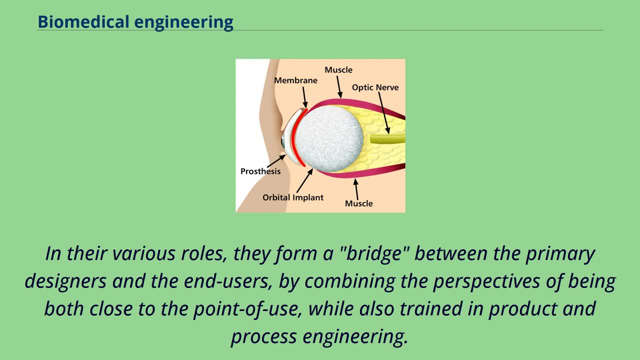 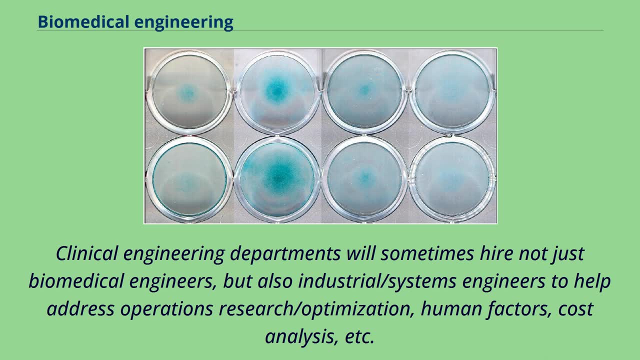 of use, while also trained in product and process engineering. Clinical engineering departments will sometimes hire not just biomedical engineers but also industrial slash systems engineers to help address operations, research, slash optimization, human factors, cost analysis, etc. Also see safety engineering for a discussion of the procedures used to design safe systems. The clinical engineering. 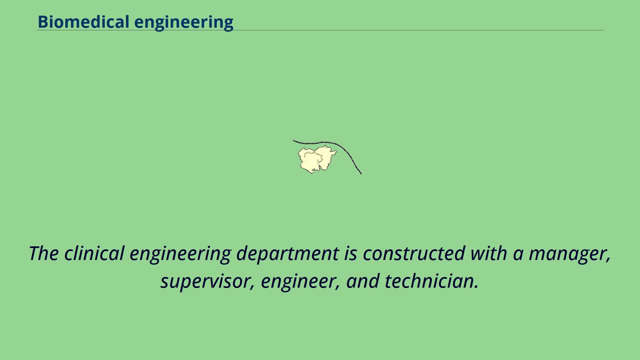 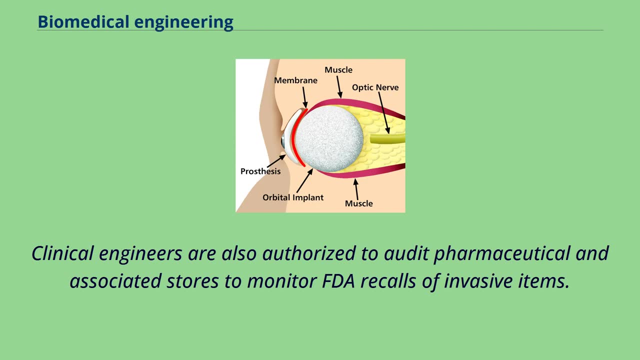 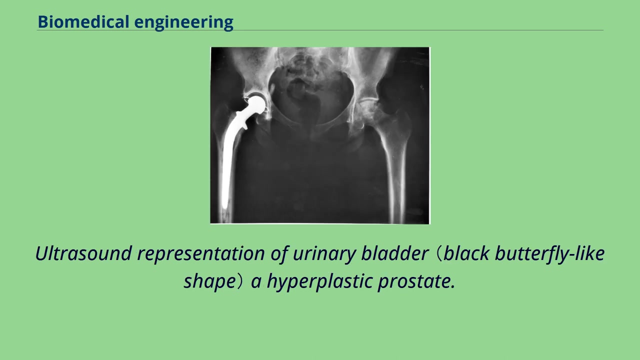 department is constructed with a manager, supervisor, engineer and technician. One engineer per 80 beds in the hospital is the ratio. Clinical engineers are also authorized to audit pharmaceutical and associated stores to monitor FDA recalls of invasive items. Ultrasound representation of urinary bladder or hyperplastic prostate- An example of practical science- and 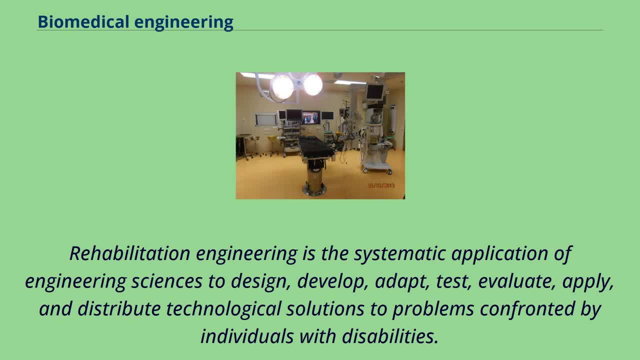 medical science working together. Rehabilitation engineering is the systematic application of engineering sciences to design, develop, adapt, test, evaluate, apply and distribute technological solutions to problems confronted by individuals with disabilities. Functional areas addressed through rehabilitation engineering may include mobility, communications, hearing, vision. 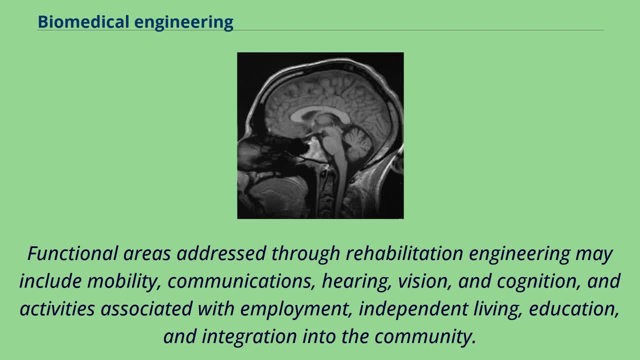 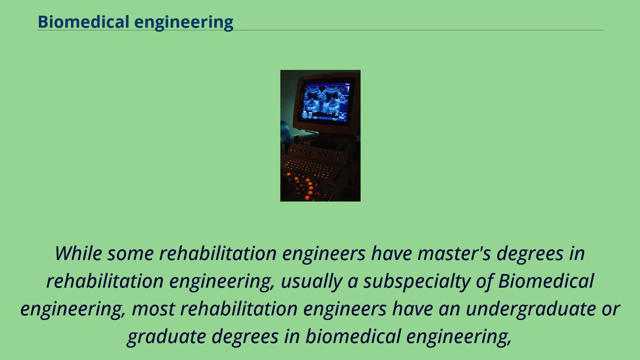 and cognition, and activities associated with employment, independent living, education and integration into the community. While some rehabilitation engineers have master's degrees in rehabilitation engineering, usually a subspecialty of biomedical engineering, most rehabilitation engineers have an undergraduate or graduate degrees in biomedical engineering. 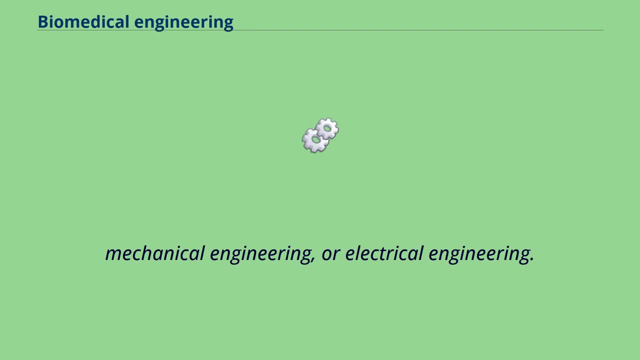 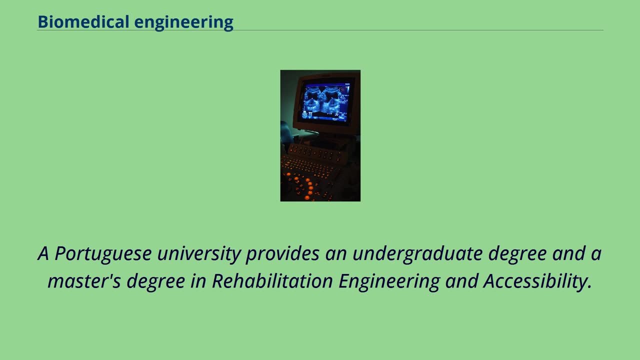 mechanical engineering or electrical engineering. A Portuguese university provides an undergraduate degree and a master's degree in rehabilitation engineering. A Portuguese university provides an undergraduate degree in rehabilitation engineering and accessibility. Qualification to become a rehab engineer in the UK is possible via a university-based say honors degree course, such 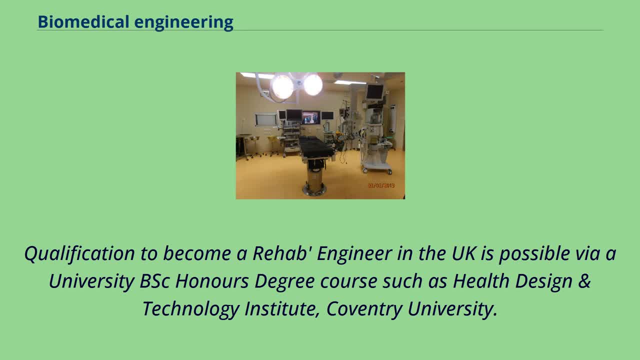 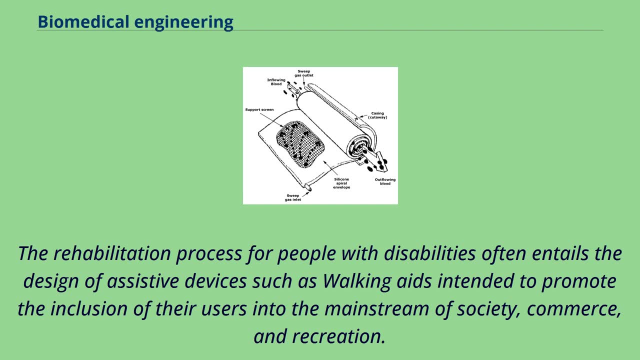 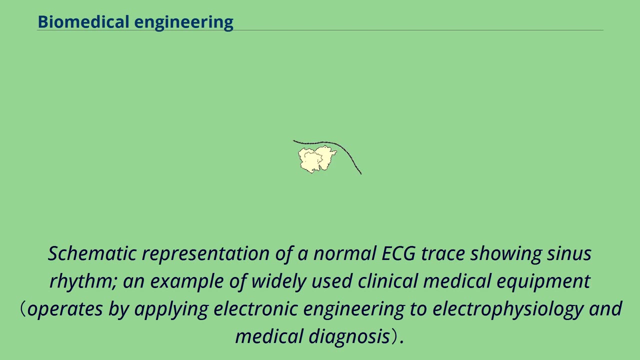 as Health Design and Technology Institute, Coventry University, The rehabilitation process for people with disabilities often entails the design of assistive devices, such as walking aids, intended to promote the inclusion of their users into the mainstream of society, commerce and recreation. Schematic representation of a normal ECG tray showing sinus rhythm, an example of walking aids and a. 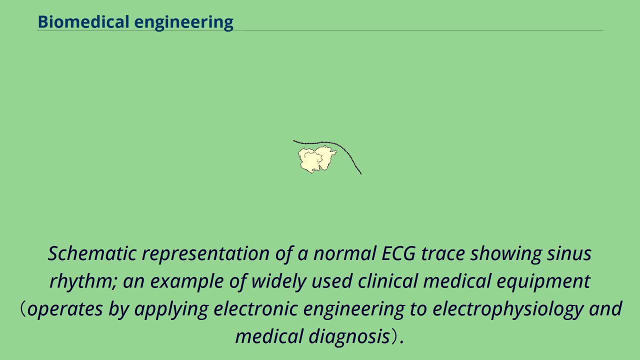 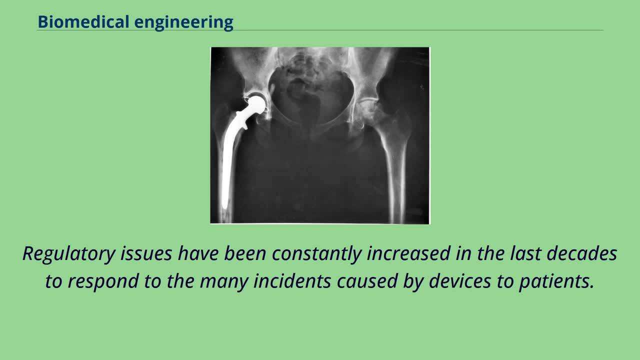 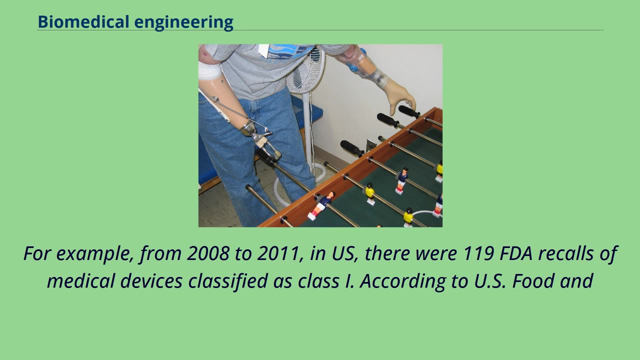 example of widely used clinical medical equipment. Regulatory issues have been constantly increased in the last decades to respond to the many incidents caused by devices to patients. For example, from 2008 to 2011,. in US, there were 119 FDA recalls of medical devices classified as Class I. according. 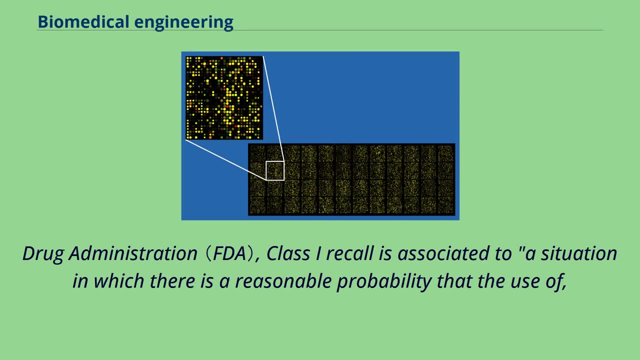 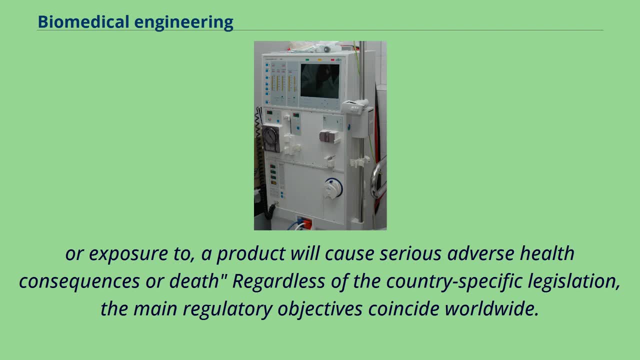 to US Food and Drug Administration Class, I recall, is associated to a situation in which there is a reasonable probability that the use of or exposure to a product will cause a disease, Serious adverse health consequences or death. regardless of the country's specific legislation, the main regulatory objectives coincide worldwide, For example in the medical device regulations. 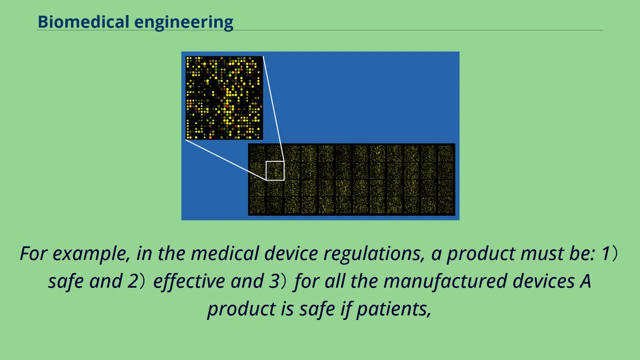 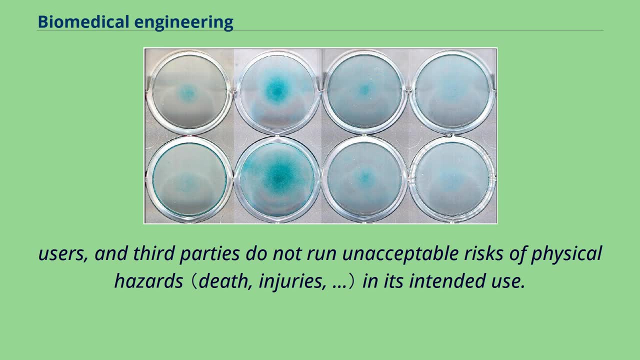 a product must be one safe and two effective, and three for all the manufactured devices. a product is safe with patients, Users and third parties do not run unacceptable risks of physical hazards in its intended use. Protective measures have to be introduced on the devices to reduce. 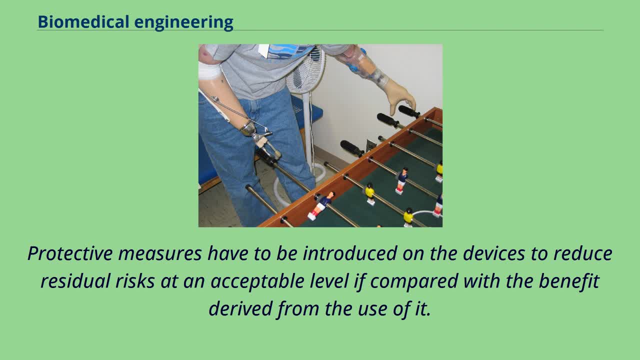 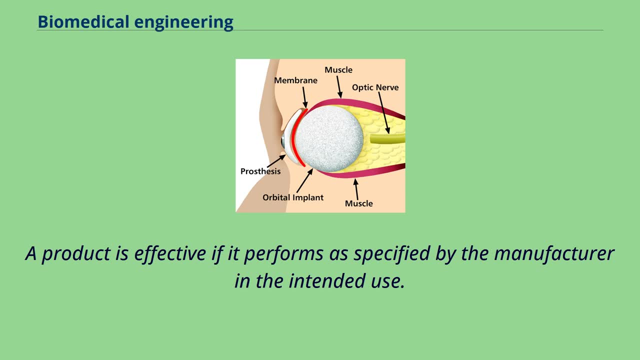 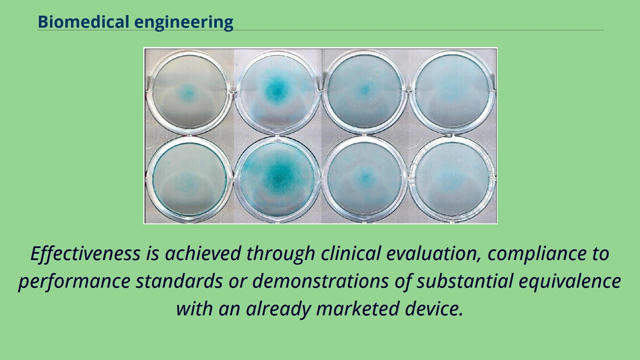 residual risks at an acceptable level If compared with the benefit derived from the use of it. a product is effective if it performs as specified by the manufacturer in the intended use. Effectiveness is achieved through clinical evaluation, compliance to performance standards or demonstrations of substantial equivalence with 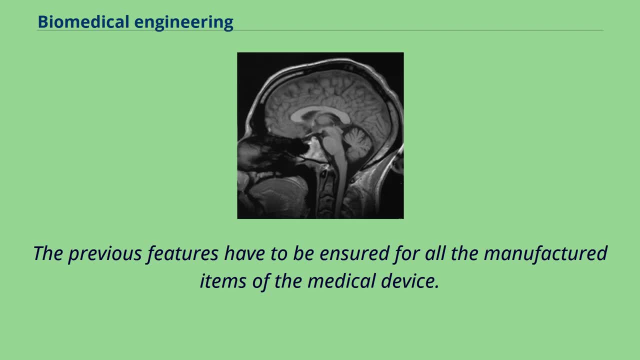 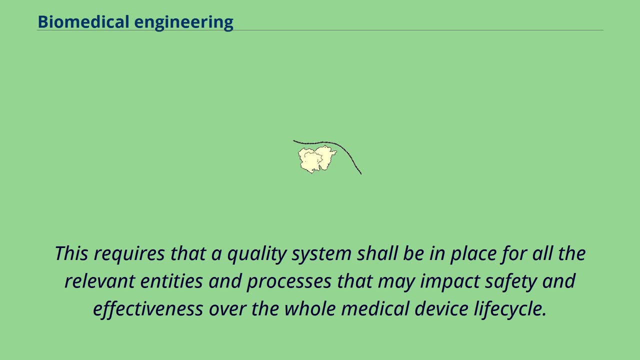 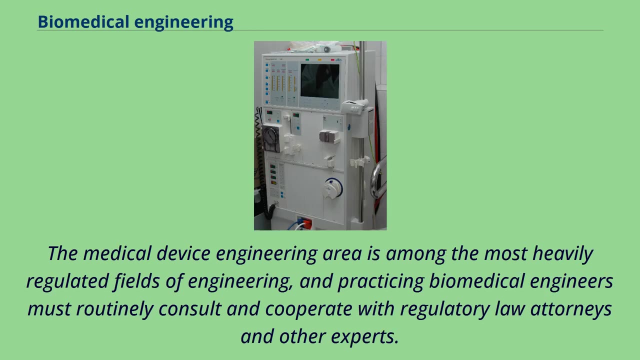 an already marketed device. The previous features have to be insured for all the manufactured items of the medical device. This requires that a quality system shall be in place for all the relevant entities and processes that may impact safety and effectiveness over the whole of the whole medical device lifecycle. The medical device engineering area is among the most heavily 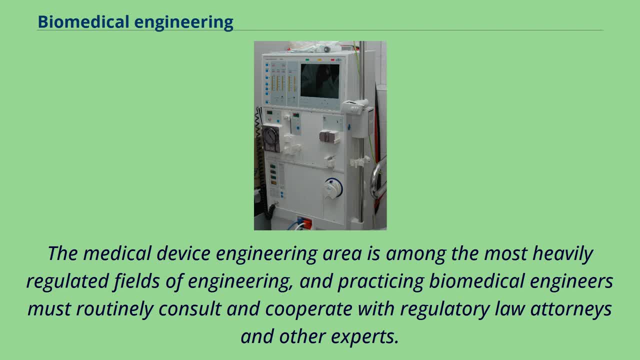 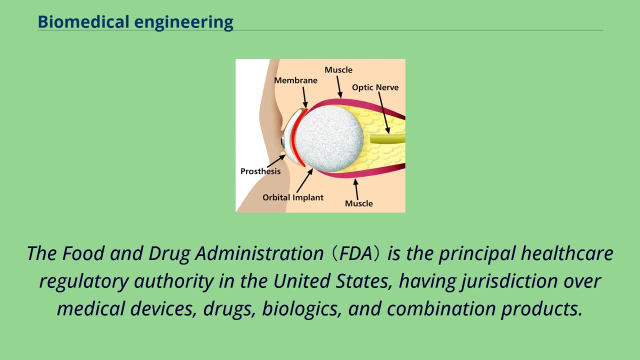 regulated fields of engineering and practicing. biomedical engineers must routinely consult and cooperate with regulatory law attorneys and other experts. The Food and Drug Administration is the principal healthcare regulatory authority in the United States, having jurisdiction over medical devices, drugs, biologics and combination products. The paramount objectives driving policy decisions. 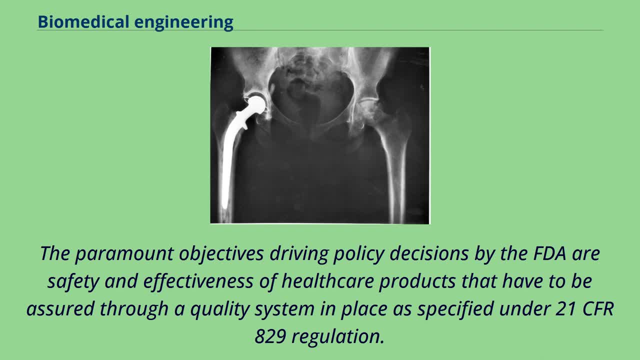 by the FDA are the following. The first is to ensure that the medical device engineering area is safety and effectiveness of healthcare products that have to be assured through a quality system in place as specified under 21 CFR 829 regulation. In addition, because biomedical engineers often 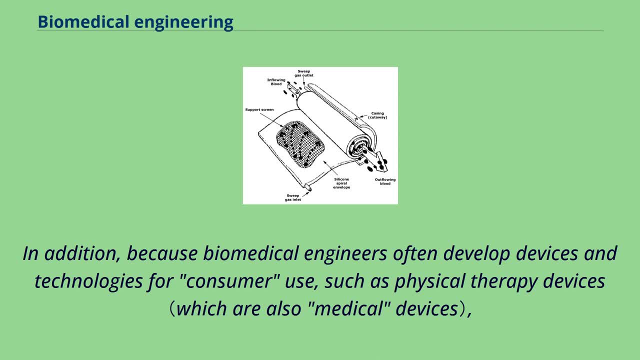 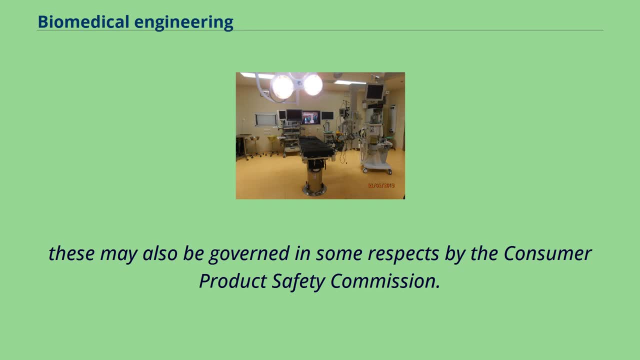 develop devices and technologies for consumer use, such as physical therapy devices. These may also be governed in some respects by the Consumer Product Safety Commission. The greatest hurdles tend to be 510k clearance or pre-market approval In the European context, safety, effectiveness and 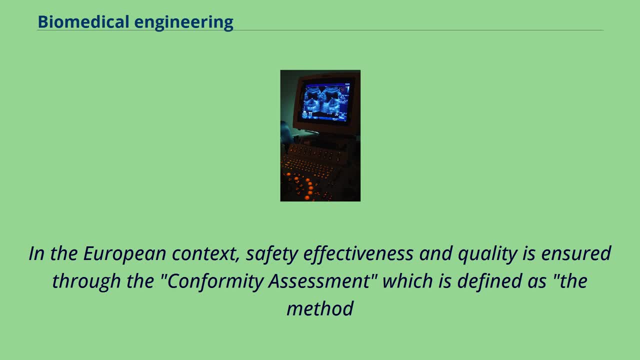 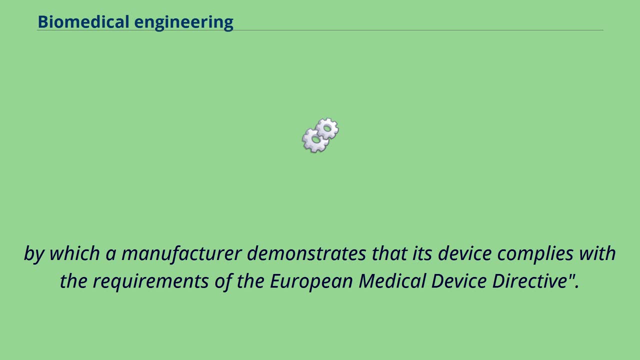 quality is ensured by the FDA. The second is to ensure that the medical device engineering area is certified through the conformity assessment, which is defined as the method By which a manufacturer demonstrates that its device complies with the requirements of the European Medical Device Directive. The directive specifies different procedures according to the class. 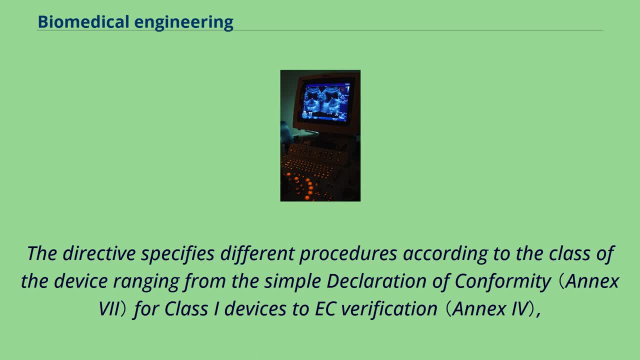 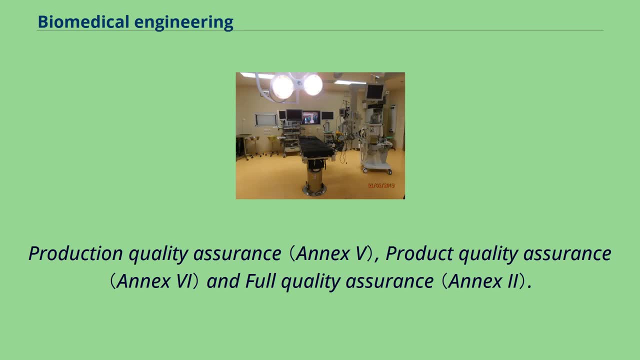 of the device, ranging from the simple declaration of conformity for class A devices to EC verification, production quality assurance, product quality assurance and full quality assurance. The medical device directive specifies detailed procedures for certification In general, the medical device engineering area is the most important part of the medical device. 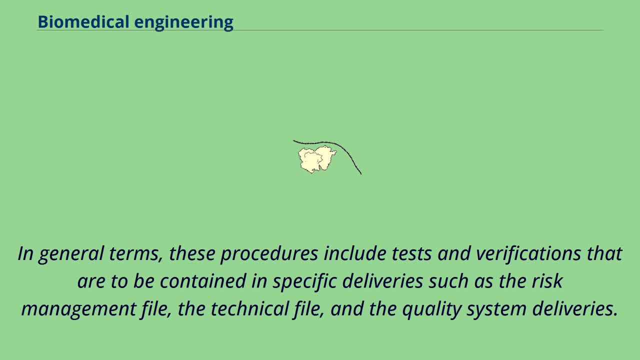 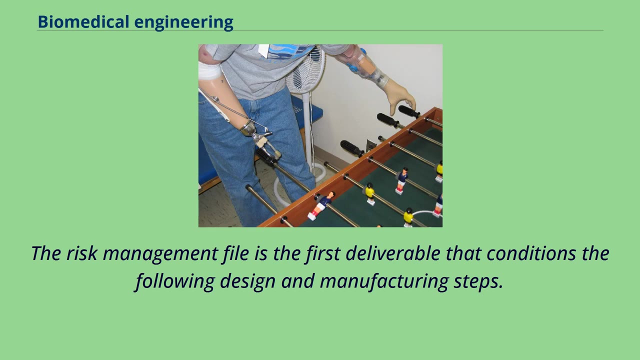 terms. These procedures include tests and verifications that are to be contained in specific deliveries, such as the risk management file, the technical file and the quality system deliveries. The risk management file is the first deliverable that conditions the following design and manufacturing steps: The risk management stage shall drive the product, so that product 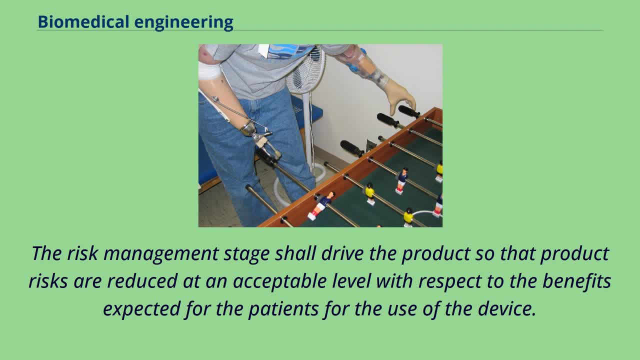 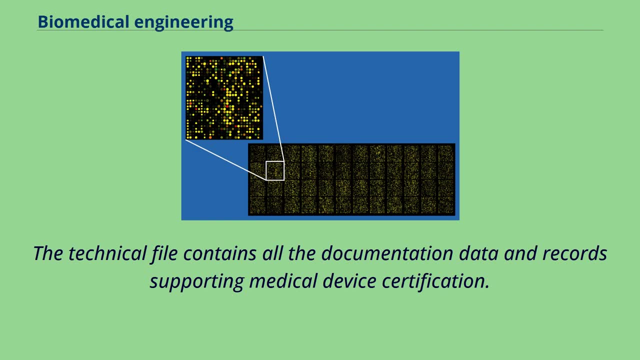 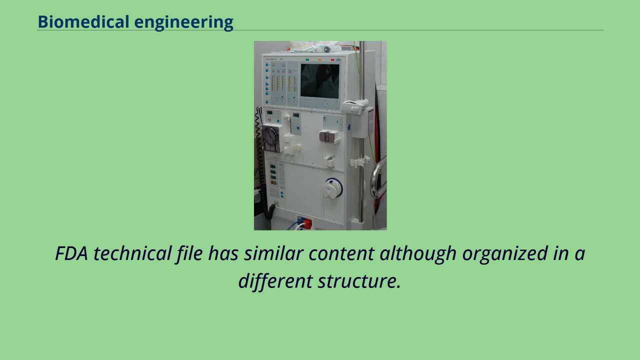 risks are reduced at an acceptable level with respect to the benefits expected for the patients for the use of the device. The technical file contains all the documentation, data and records supporting medical device certification. FDA technical file has similar content, although organized in a different structure. The quality system deliverables usually include procedures. 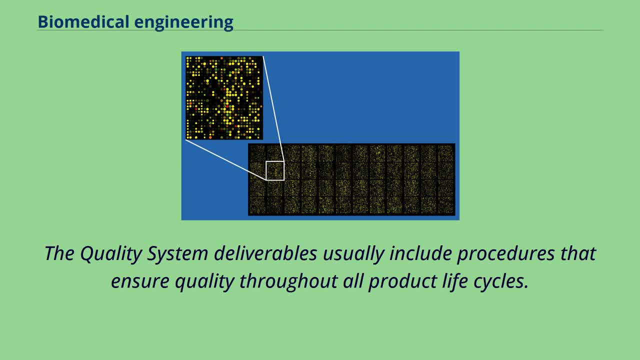 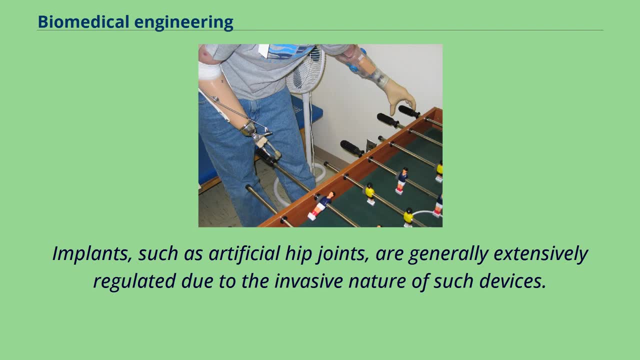 that ensure quality throughout all product life cycles. The same standard is usually applied for quality management systems in the US and worldwide. Implants such as artificial hip joints are generally extensively regulated due to the invasive nature of such devices. In the European Union there are certifying entities. 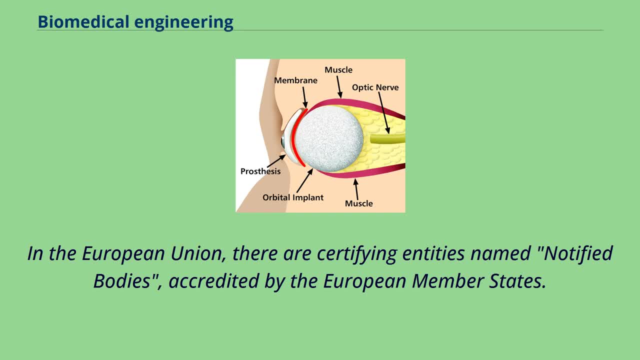 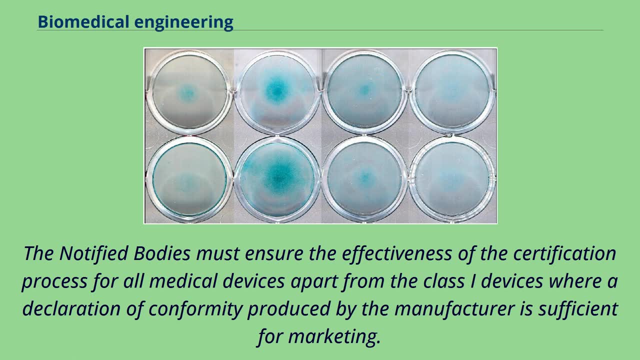 Notified bodies must ensure the effectiveness of the certification process for all medical devices apart from the class I devices, where a declaration of conformity produced by the manufacturer is sufficient for marketing. Once a product has passed all the steps required by the medical device directive, the device is entitled to bear a CE marking indicating that. 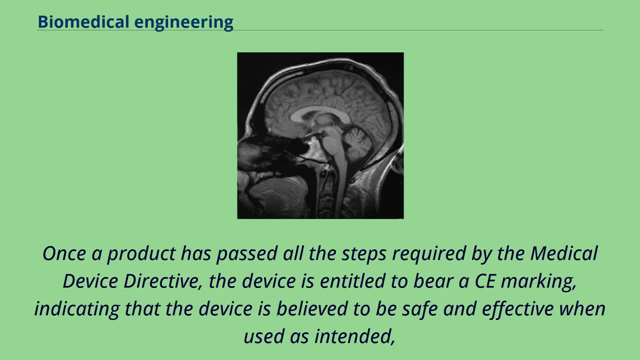 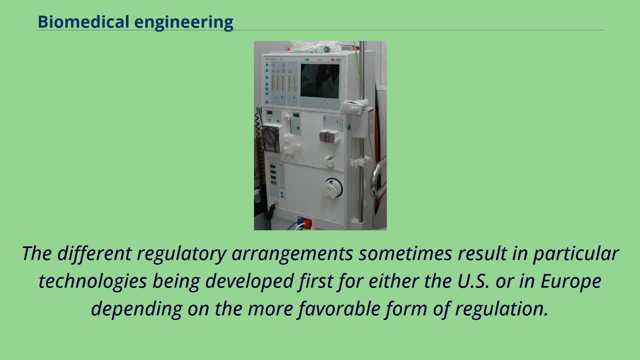 the device is believed to be safe and effective when used as intended And therefore it can be marketed within the European Union. The medical device must ensure the effectiveness of the certification process in the European Union. The different regulatory arrangements sometimes result in particular technologies being developed first for either the US or in Europe, depending on 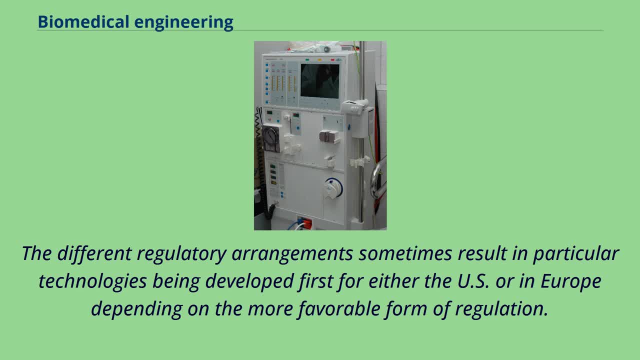 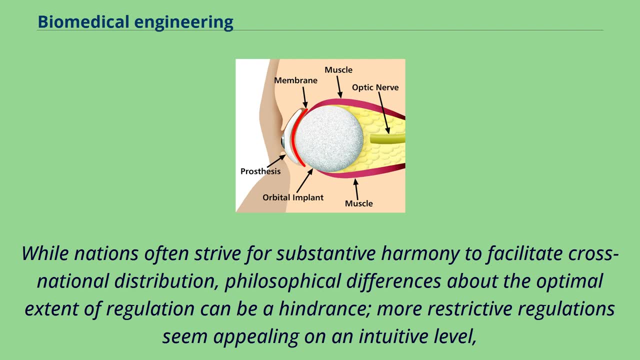 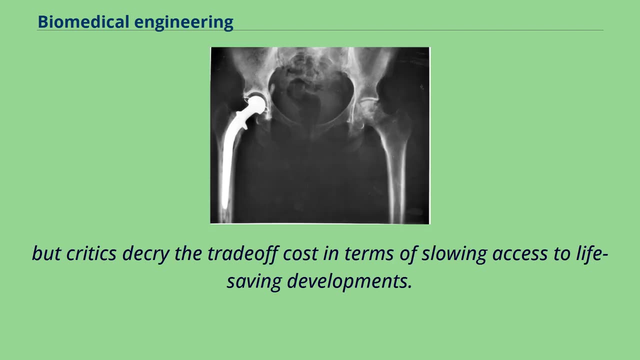 the more favorable form of regulation. While nations often strive for substantive harmony to facilitate cross-national distribution, philosophical differences about the optimal extent of regulation can be a hindrance. More restrictive regulations seem appealing on an intuitive level, But critics decry the trade-off cost in terms of slowing access to life-saving. 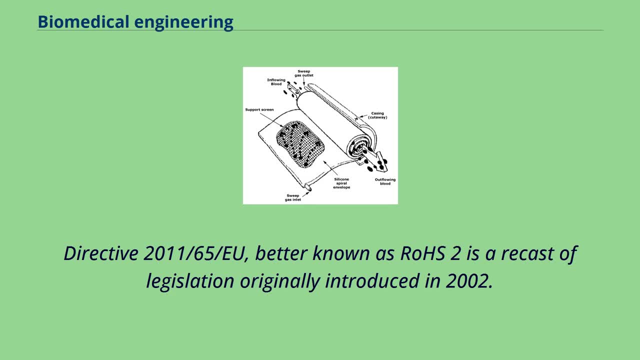 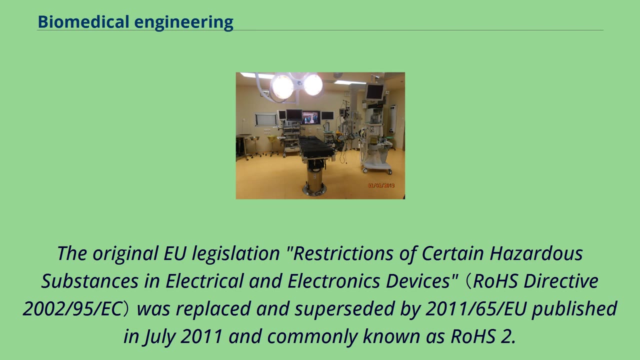 developments. Directive 2011-65-EU, better known as RHO-HS-2, is a recast of legislation originally introduced in 2002.. The original EU legislation restrictions of certain hazardous substances in electrical and electronics devices was replaced and superseded by 2011-65-EU, published in July 2011 and commonly. 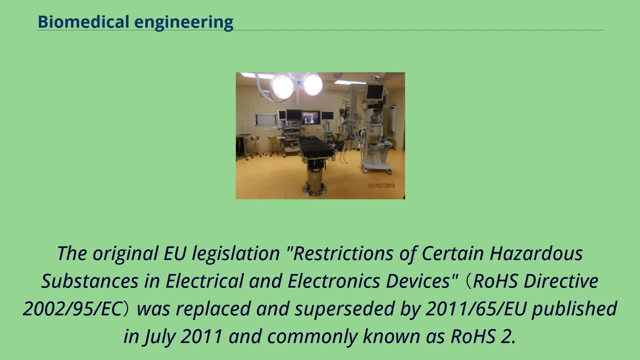 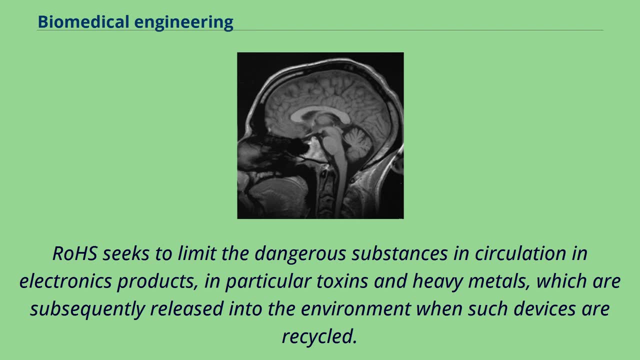 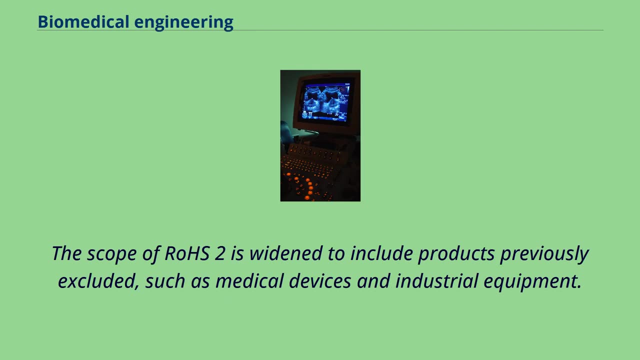 known as RHO-HS-2.. RHO-HS seeks to limit the dangerous substances in circulation in electronics products. in particular, toxin RHO-HS-2 is designed to reduce the risk of damage to the environment when such devices are recycled. The scope of RHO-HS-2 is widened to include products previously excluded. 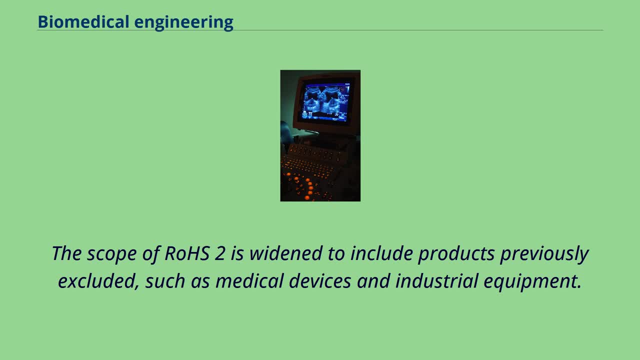 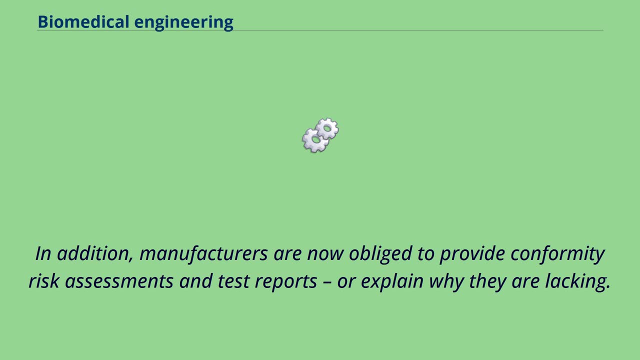 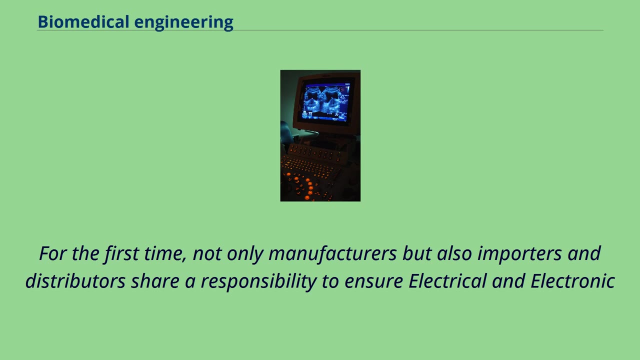 such as medical devices and industrial equipment. In addition, manufacturers are now obliged to provide conformity risk assessments and test reports or explain why they are lacking. For the first time, not only manufacturers, but also importers and distributors share a responsibility to ensure electrical and electronic 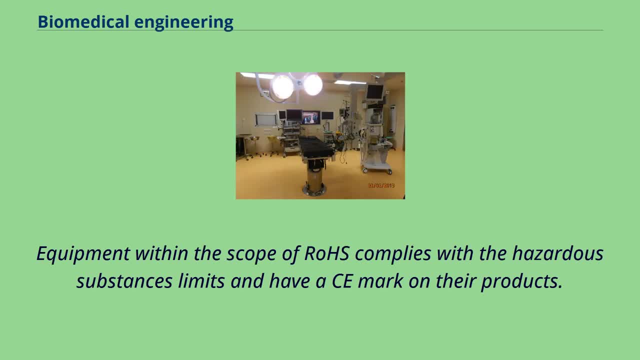 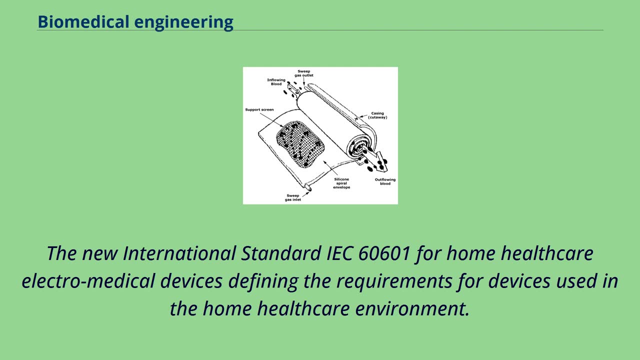 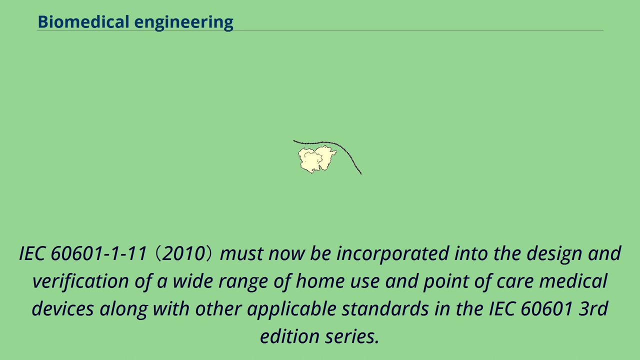 equipment within the scope of RHO-HS-2.. RHO-HS-2 is designed to reduce the risk of damage to the environment only when such devices are affected. The mandatory date for implementation of the N-European version of the standard is June 1,. 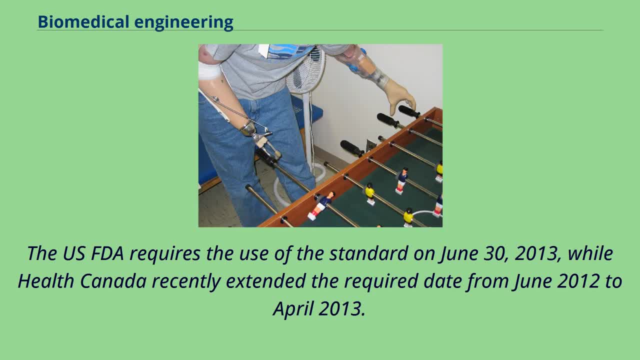 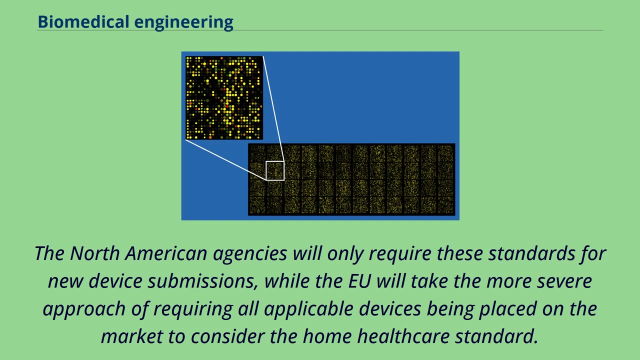 2013.. The US FDA requires the use of the standard on June 30, 2013,, while Health Canada recently extended the required date from June 2012 to April 2013.. The North American agencies will only require these standards for new device submissions, while the EU will take the more. 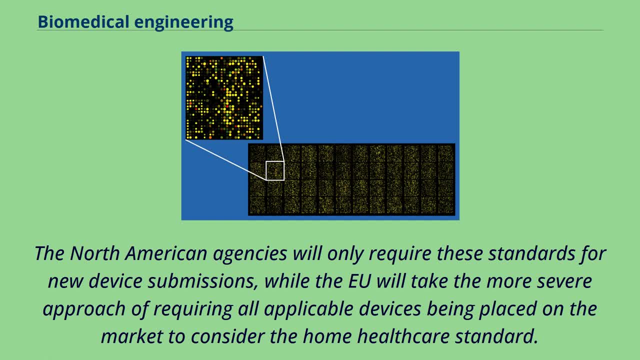 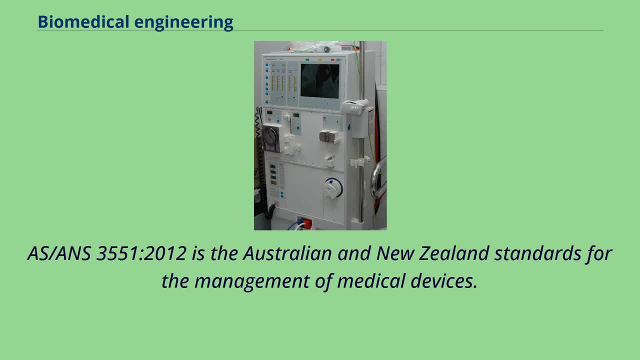 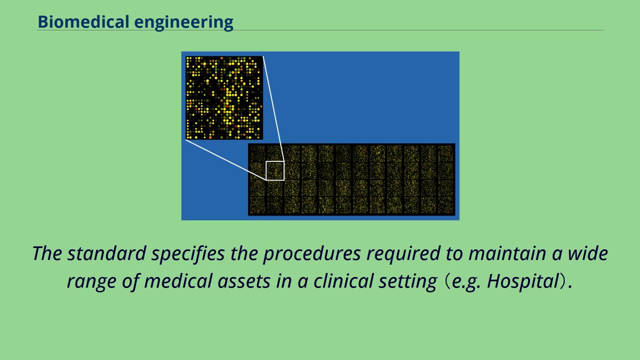 severe approach of requiring all applicable devices being placed on the market to consider the home healthcare standard. AS-ANS 3551-2012 is the Australian and New Zealand standards for the management of medical devices. The standard specifies the procedures required to maintain a 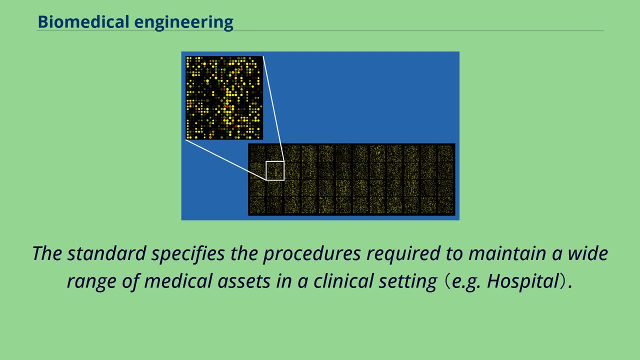 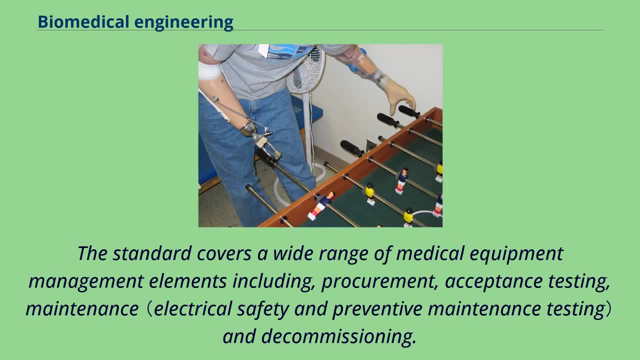 wide range of medical assets in a clinical setting. The standards are based on the IEC 606101 standards. The standard covers a wide range of medical equipment management elements, including procurement, acceptance, testing, maintenance and decommissioning. Biomedical engineers require considerable knowledge of both engineering and biology. 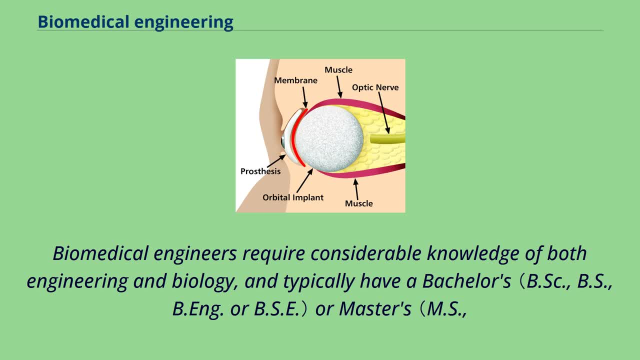 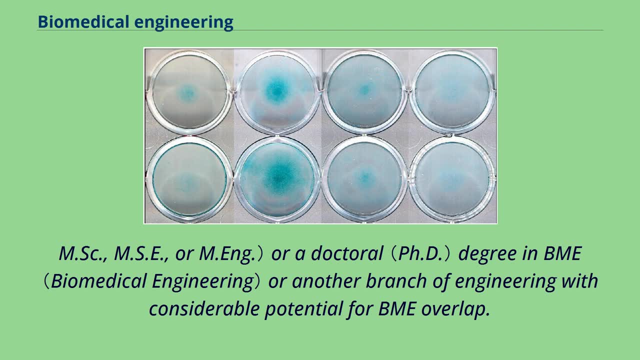 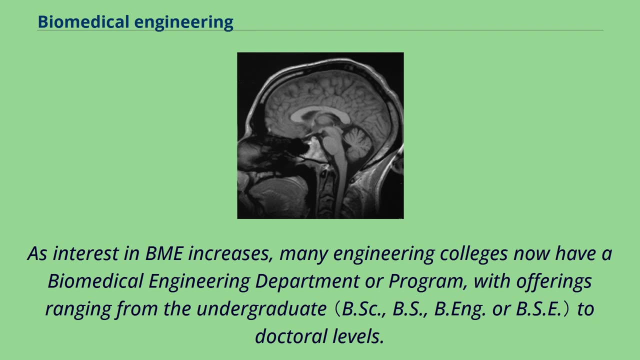 and typically have a bachelor's or master's, MS, MSc, MSE or Master of Engineering or a doctoral degree in BME or another branch of engineering with considerable potential for BME overlap As interest in BME increases. many engineering colleges now have a biomedical engineering. 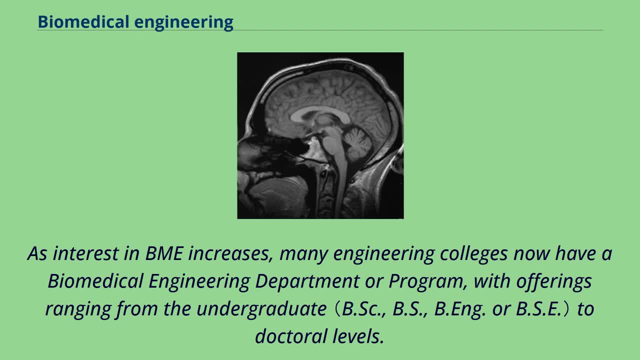 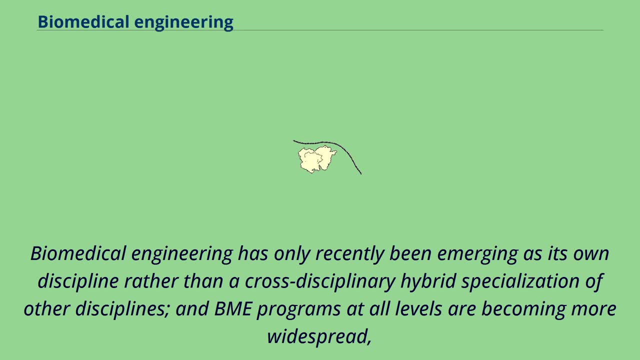 department or program, with offerings ranging from the undergraduate to doctoral levels. Biomedical engineering has only recently been emerging as its own discipline rather than a cross-disciplinary hybrid specialization of other disciplines, and BME programs at all levels are becoming more widespread, Including the Bachelor of Science in Biomedical Engineering, which includes enough biological. 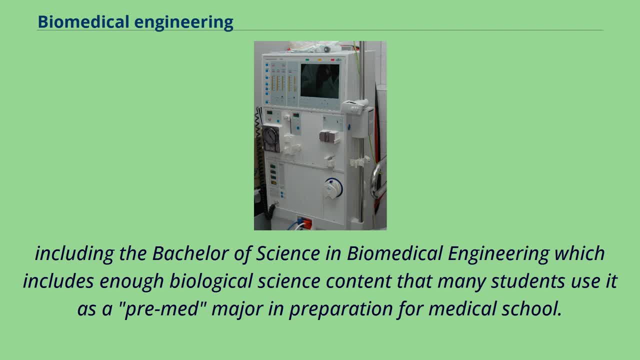 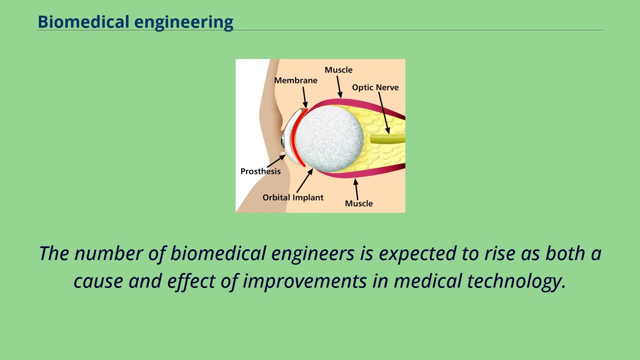 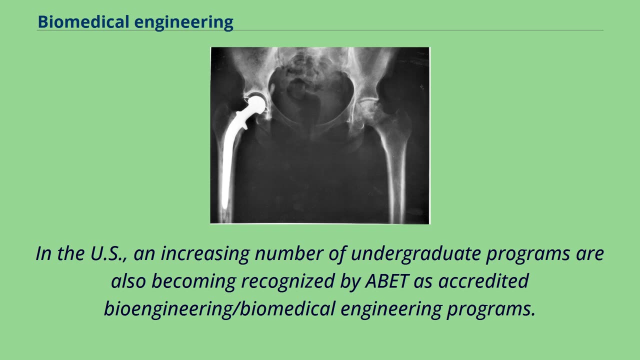 science content that many students use it as a pre-med major in preparation for medical school. The number of biomedical engineers is expected to rise as both a cause and effective improvements in medical technology. In the US, an increasing number of undergraduate programs are also becoming recognized by ABET as accredited bioengineering slash- biomedical engineering. 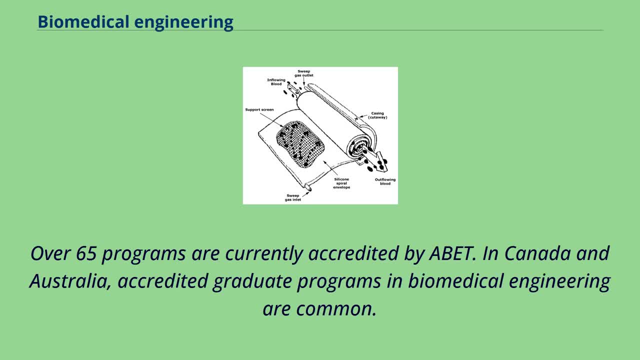 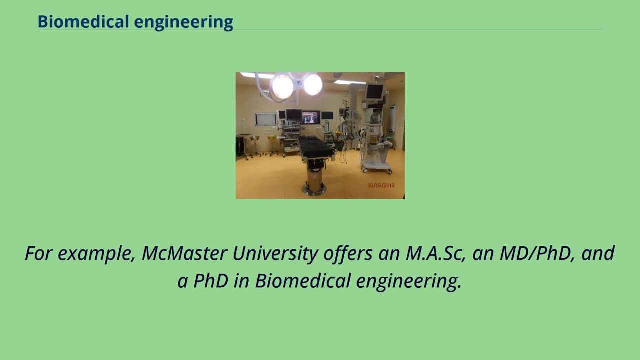 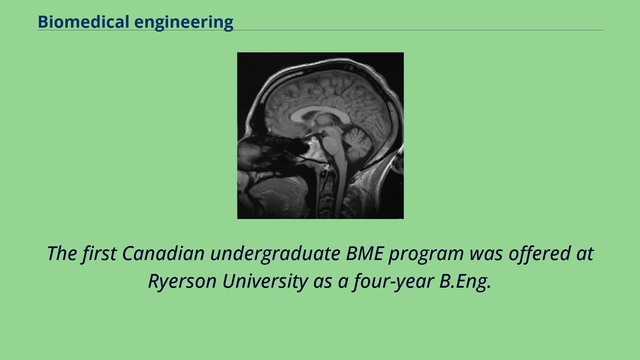 programs. Over 65 programs are currently accredited by ABET. In Canada and Australia, accredited graduate programs in biomedical engineering are common. For example, McMaster University offers an MASC, an MD, slash PhD and a PhD in biomedical engineering. The first Canadian undergraduate BME program was offered at Ryerson University as a four-year BA. 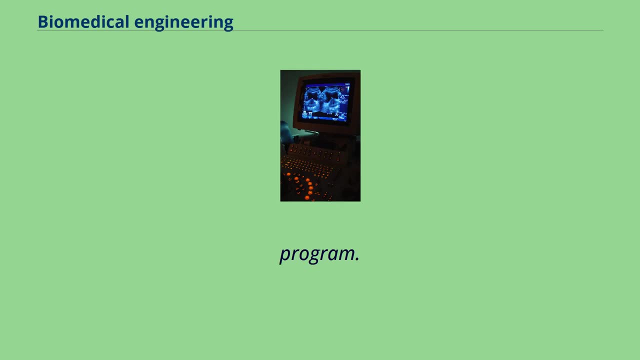 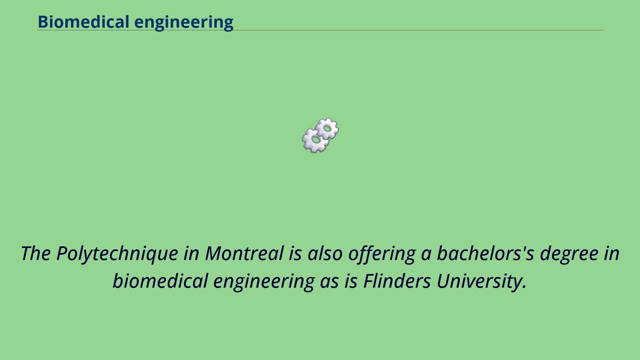 program. The Polytechnique in Montreal is also offering a bachelor's degree in biomedical engineering, as is Flinders University. As with many degrees, the reputation and ranking of a program may factor into the desirability of a degree holder for either employment or graduate admission. 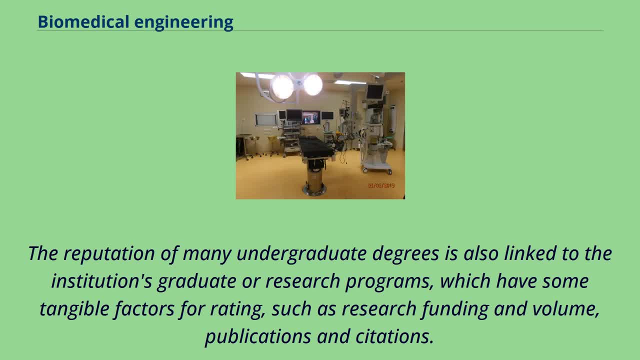 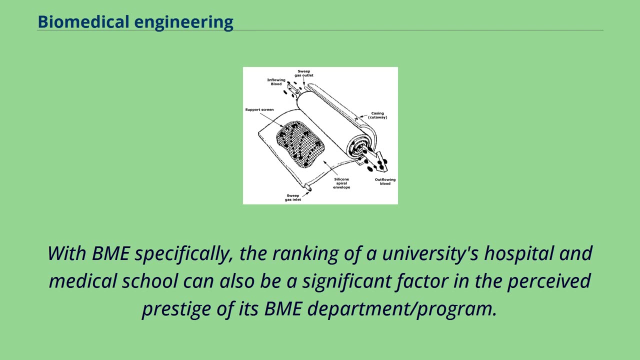 The reputation of many undergraduate degrees is also linked to the institution's graduate or research programs, which have some tangible factors for rating, such as research funding and volume, publications and citations. BME, specifically the ranking of a university's hospital and medical school, can also be a. 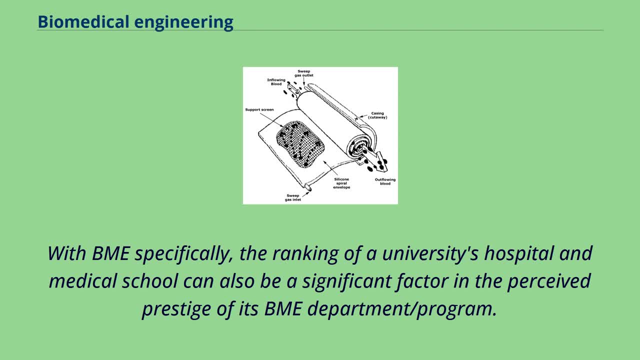 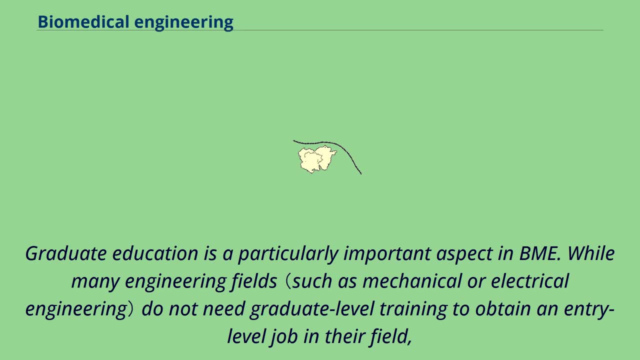 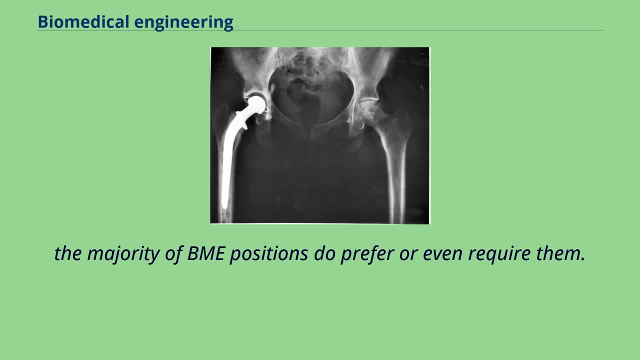 significant factor in the perceived prestige of its BME department slash program. Graduate education is a particularly important aspect in BME. While many engineering fields do not need graduate-level training to obtain an entry-level job in their field, the majority of BME positions do prefer or even require them, Since most BME-related professions involve 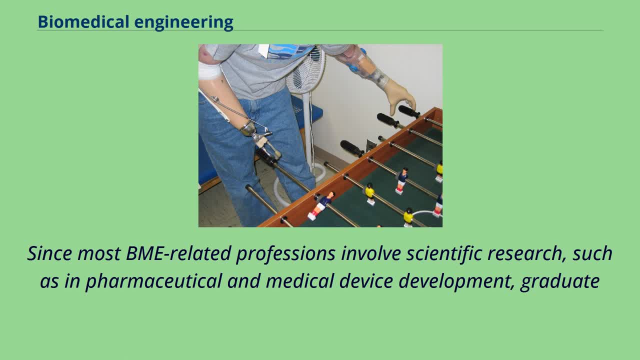 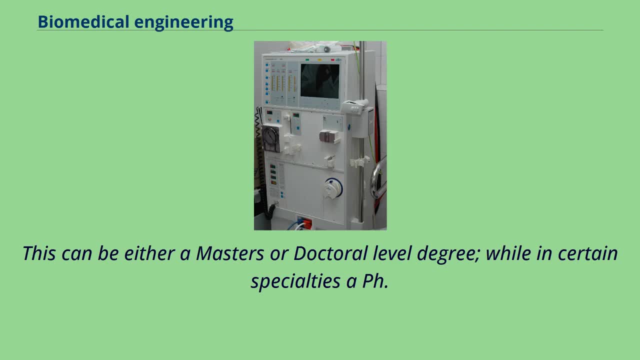 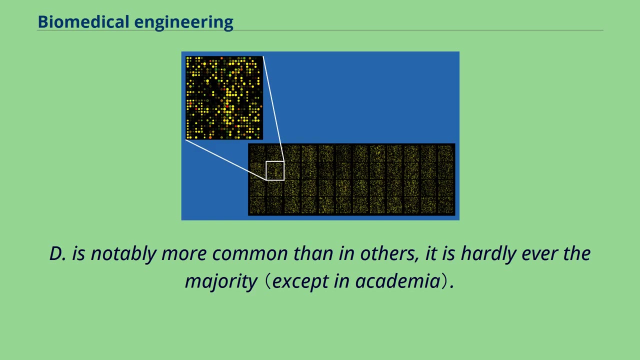 scientific research, such as in pharmaceutical and medical device development, graduate education is almost a requirement. This can be either a master's or doctoral-level degree. while in certain specialties a Ph D is notably more common than in others, it is hardly ever- the majority, In fact- the perceived need for some kind of graduate. 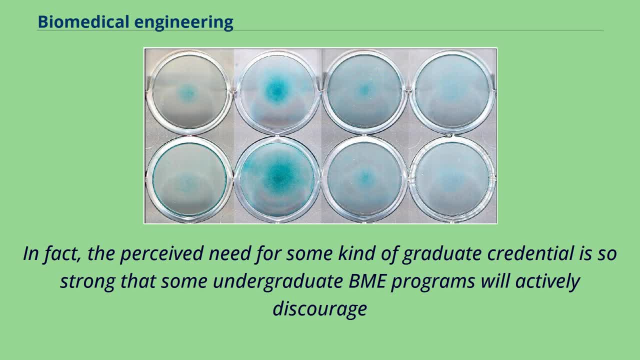 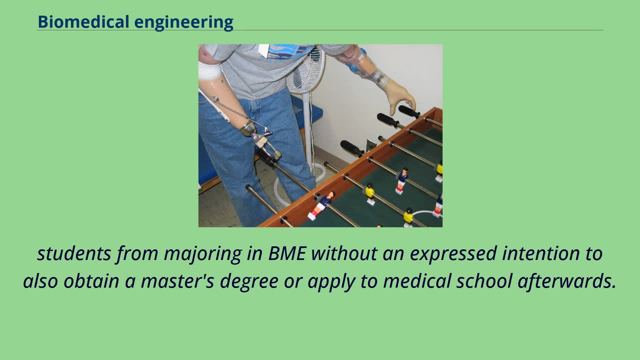 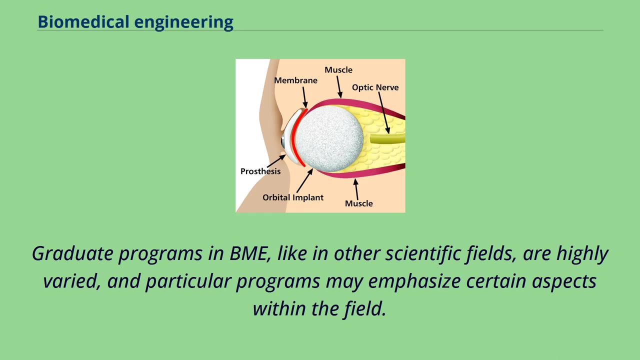 credential is so strong that some undergraduate BME programs will actively discourage students from majoring in BME without an expressed intention to also obtain a master's degree or apply to medical school afterwards. Programs in BME, like in other scientific fields, are highly varied and particular. 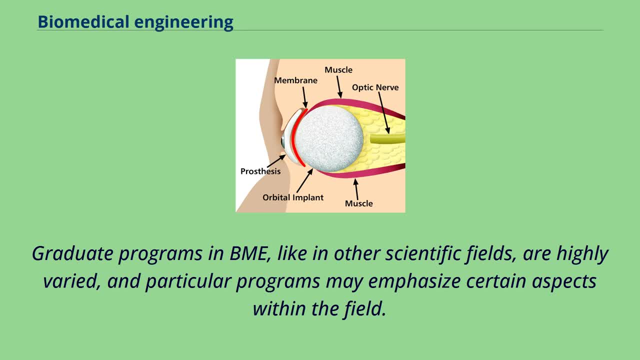 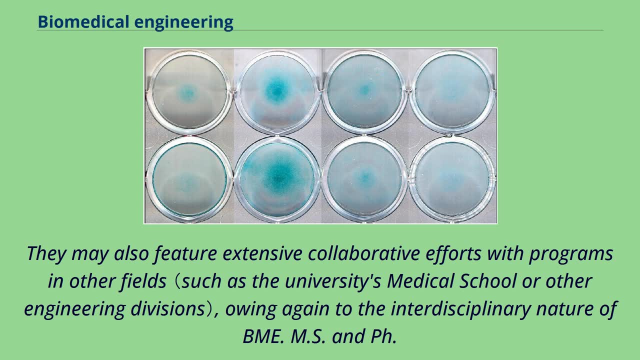 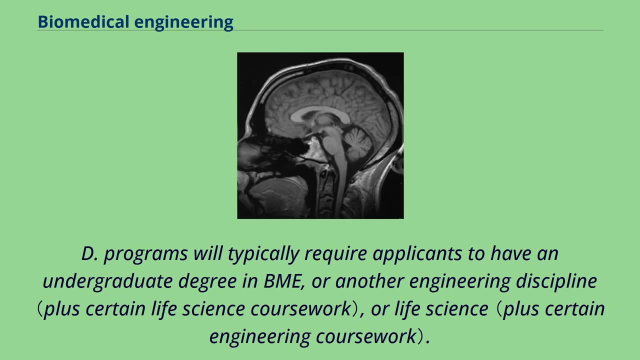 programs may emphasize certain aspects within the field. They may also feature extensive collaborative efforts with programs in other fields. owing again to the interdisciplinary nature of BME, MS and Ph D programs will typically require applicants to have an undergraduate degree in BME or another engineering discipline or life science. 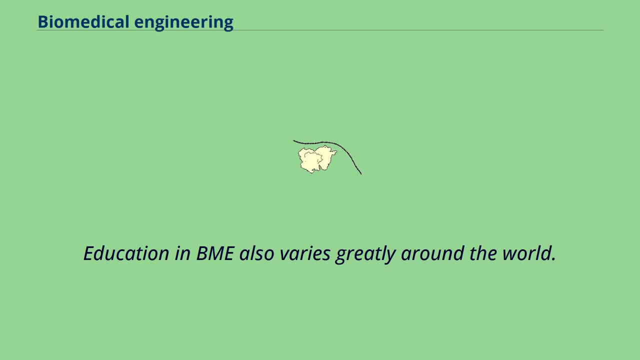 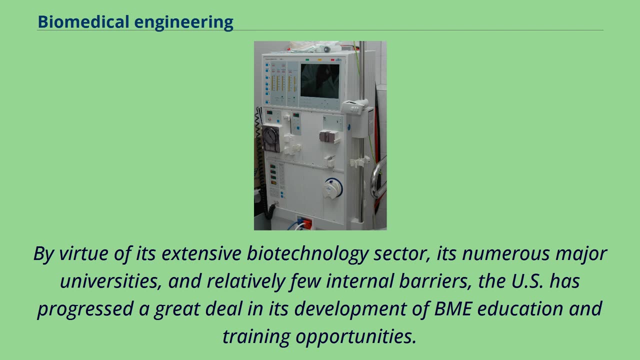 Education in BME also varies greatly around the world. By virtue of its extensive biotechnology sector, its numerous major universities and relatively few internal barriers, the US has progressed a great deal in its development of BME education and training opportunities. Europe, which also has a large biotechnology sector and an impressive 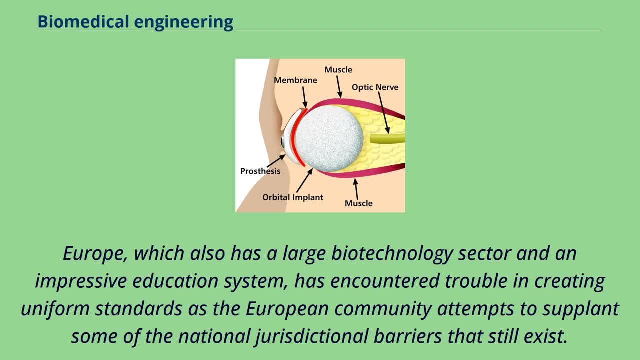 education system has encountered trouble in creating uniform standards as the European community attempts to supplant some of the national jurisdictional barriers that still exist. Recently, initiatives such as Biomedia have sprung up to develop BME research and development, and the US has begun to develop BME research and development. 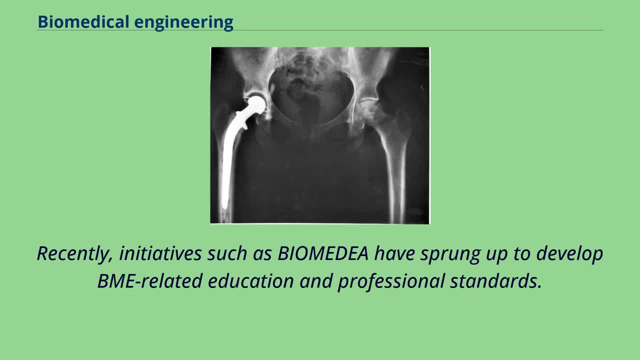 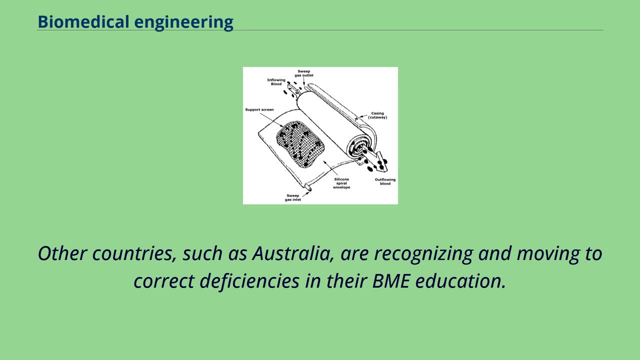 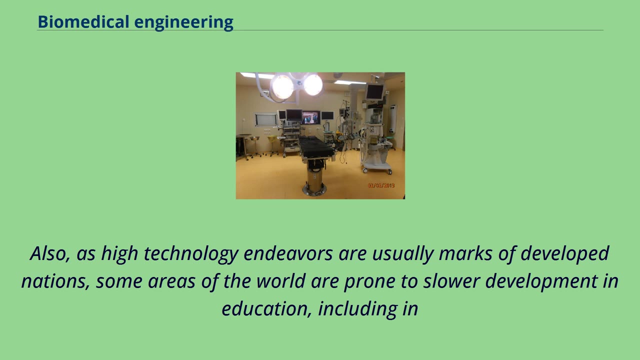 Other countries, such as Australia, are recognizing and moving to correct deficiencies in their BME education. Also, as high technology endeavors are usually marks of developed nations, some areas of the world are prone to slower development in education, including in BME. As with other learned professions, each state has certain requirements for becoming 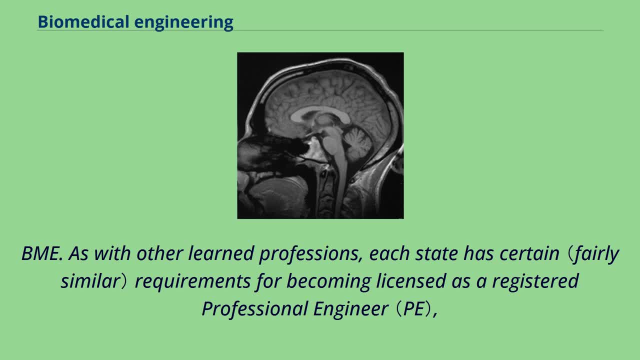 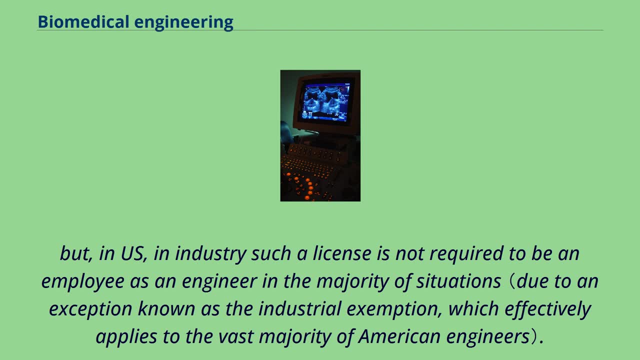 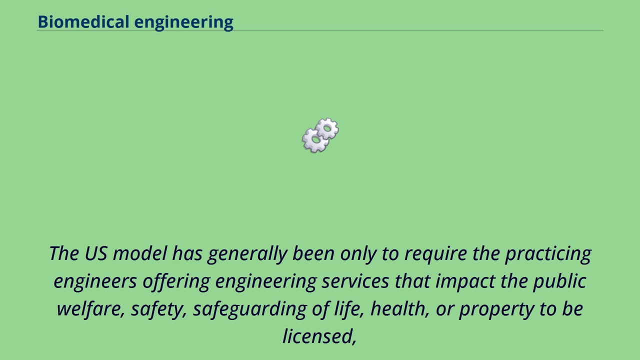 licensed as a registered professional engineer, But in US, in industry, such a license is not required. The US model has generally been only to require the practicing engineers offering engineering services that impact the public: welfare, safety, safeguarding of life, health. 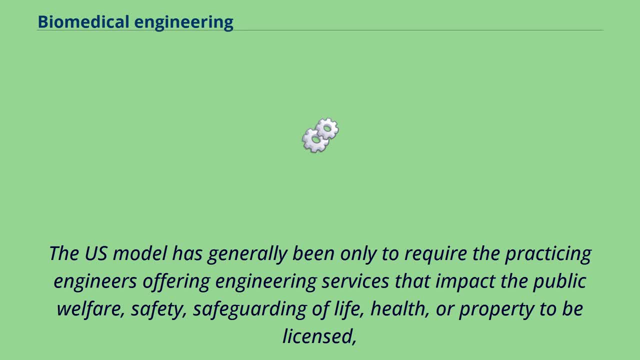 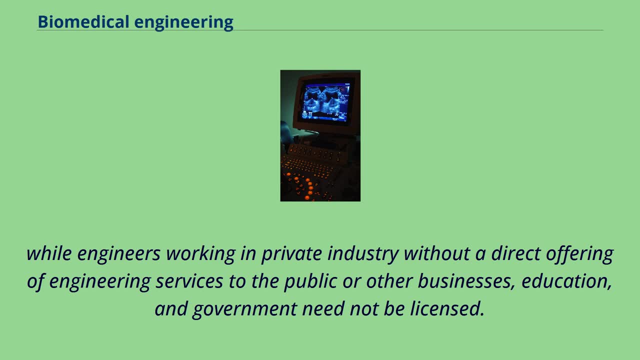 or property to be licensed, While engineers working in private industry without a direct offering of engineering services to the public or other businesses, education and government need not be licensed. This is notably not the case in many other countries where a license is as 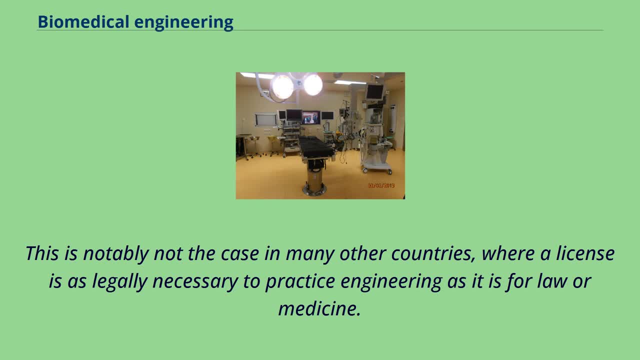 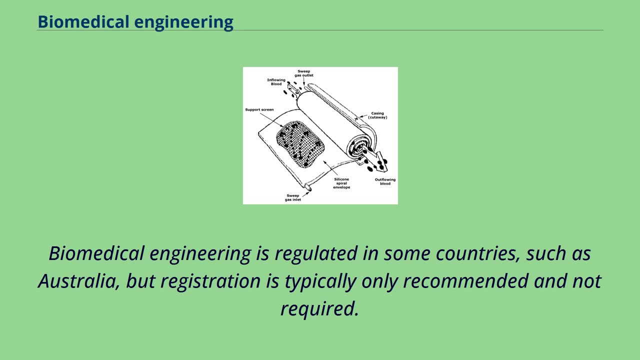 legally necessary as a registered professional engineer. The US model has generally been only necessary to practice engineering, as it is for law or medicine. Biomedical engineering is regulated in some countries such as Australia, but registration is typically only recommended and not required In the UK. mechanical engineers working in the areas of medical 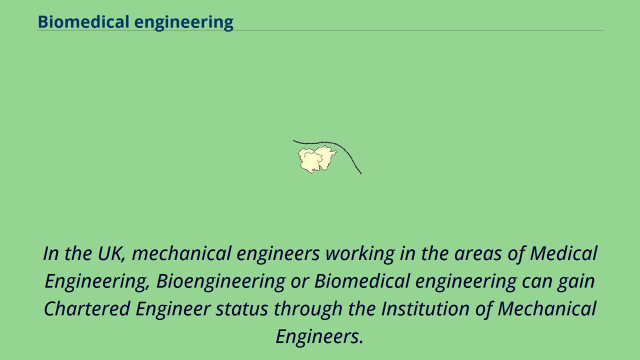 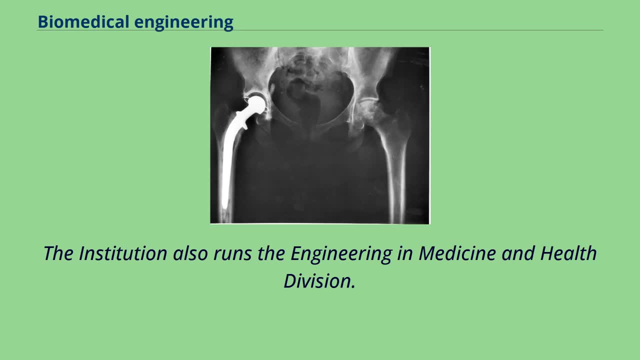 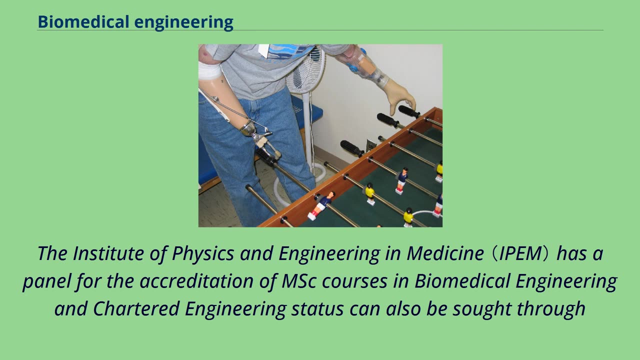 engineering, bioengineering or biomedical engineering can gain chartered engineer status through the Institution of Mechanical Engineers. The institution also runs the Engineering and Medicine and Health Division. The Institute of Physics and Engineering and Medicine has a panel for the accreditation of MSc courses in biomedical engineering and chartered engineering status can. 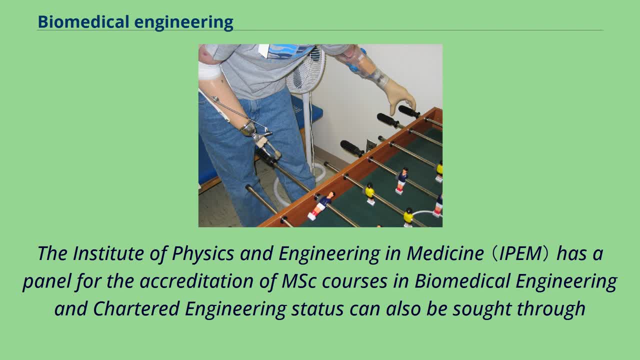 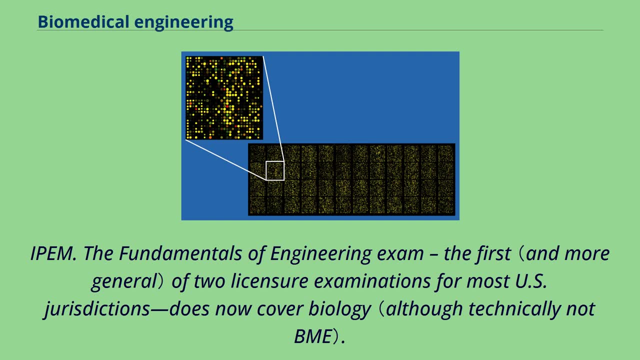 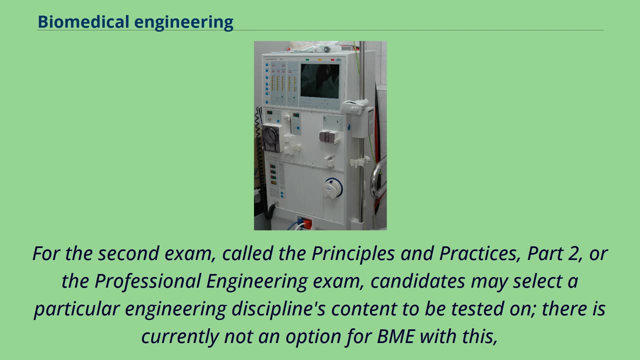 also be sought through IPEAM. The Fundamentals of Engineering Exam, the first of two licensure examinations for most US jurisdictions does now cover biology. For the second exam, called the Principles and Practices Part 2, or the Professional Engineering Exam, candidates may select a particular. 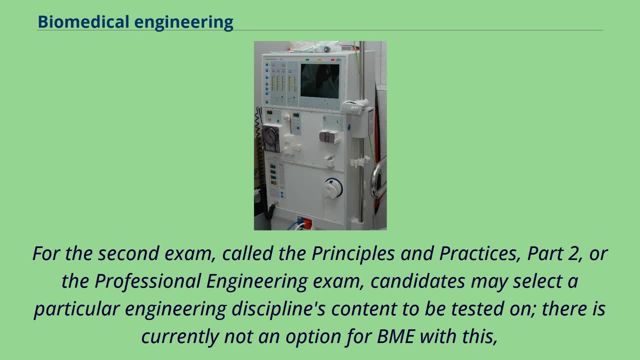 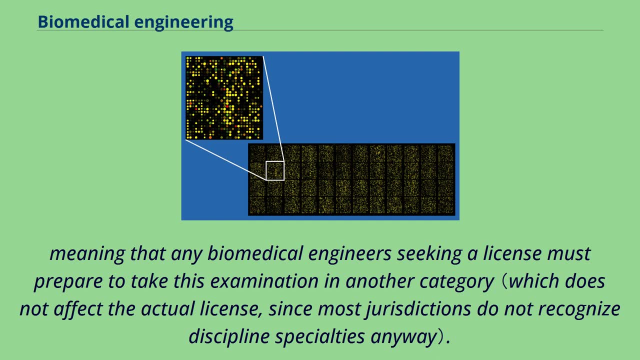 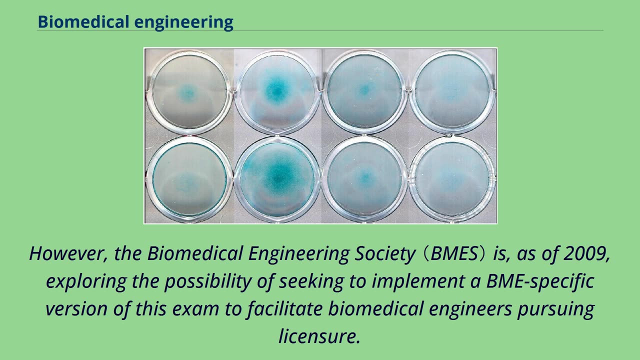 engineering disciplines content to be tested on. There is currently not an option for BME with this. Any biomedical engineer seeking a license must prepare to take this examination. in another category, However, the Biomedical Engineering Society is, as of 2009,, exploring the possibility. 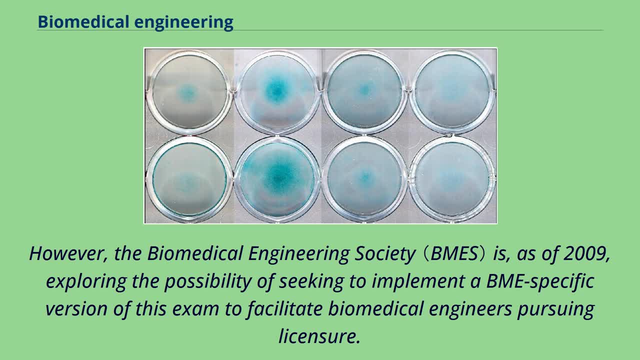 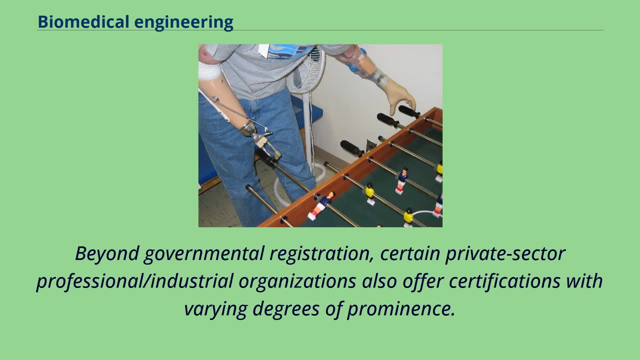 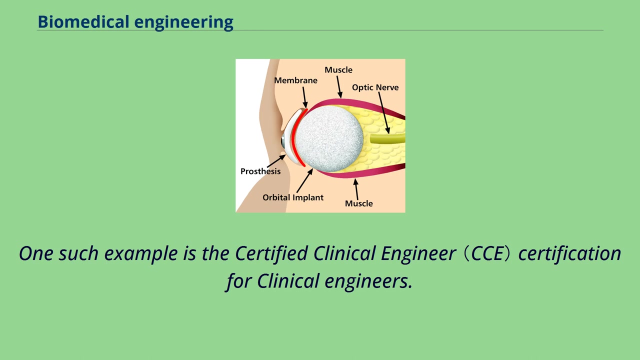 of seeking to implement a BME-specific version of this exam to facilitate biomedical engineers pursuing licensure Beyond governmental registration. certain private sector professional-slash-industrial organizations also offer certifications with varying degrees of prominence. One such example is the Certified Clinical Engineer Certification for Clinical Engineers. 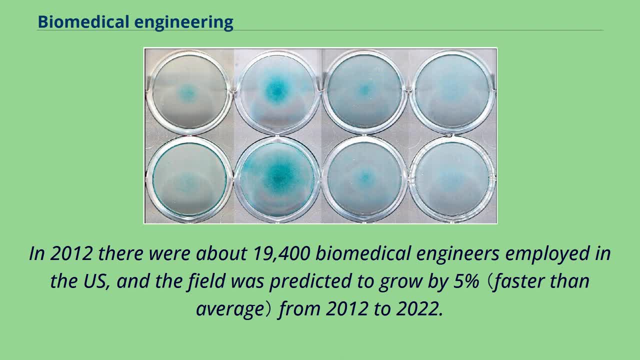 In 2012, there were about 19,400 biomedical engineers employed in the US, and the field was predicted to grow by 5% from 2012 to 2022.. Biomedical engineering has the highest percentage of female engineers compared to other common engineering professions.